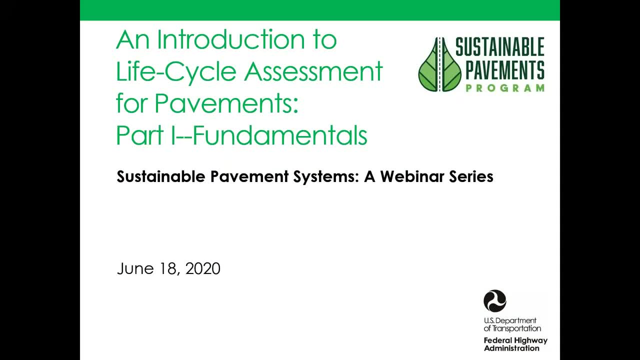 Good afternoon everyone and welcome to the webinar. My name is Kurt Smith, with Applied Pavement Technology, and I'll be serving as your host for today's webinar on an Introduction to Lifecycle Assessment for Pavements: Part 1- Fundamentals. This is part of an ongoing 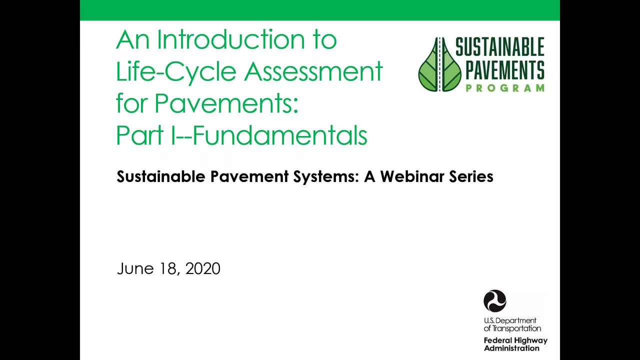 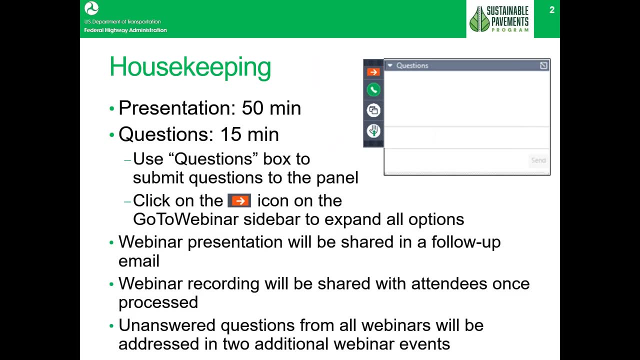 series of webinars on sustainability that were developed under the FHWA's Sustainable Pavements Program and covers all stages of the pavement lifecycle. Before we get started here today, I want to mention just a few housekeeping items. The webinar itself is scheduled for. 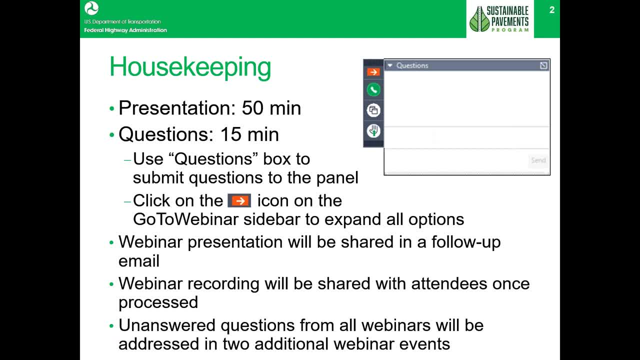 a total of one hour and consists of a 50-minute formal presentation and a 10-minute question and answer session. The questions will be answered at the end of the formal presentation, but you may submit your questions at any time during the presentation using the questions. 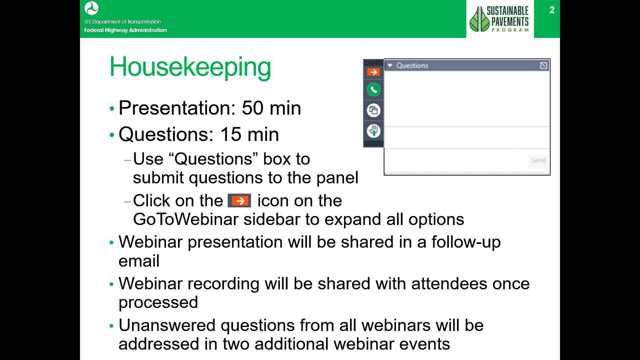 box. If you don't see the questions box, you may need to click on the orange arrow icon on the control panel to display the settings At the end of the session. we will work to answer as many of the questions as we can within the time allotted, but because of the 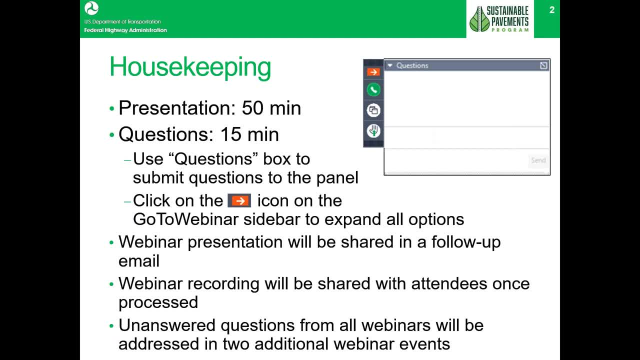 volume of questions, we likely will not be able to get through all of them. However, currently plans are being made to organize two additional webinar events to address all of the questions that have been raised on all of the webinars. If you have any questions about any of the questions that have been raised on all of 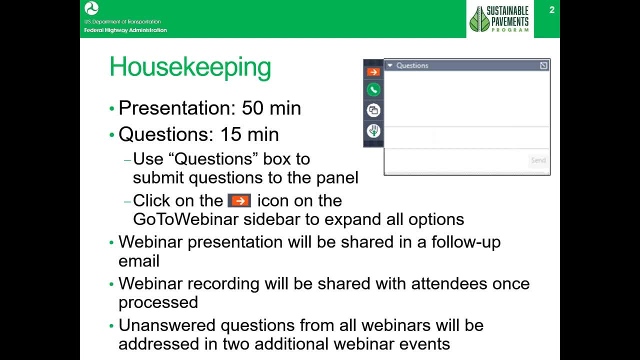 the past webinar session events. details on those additional webinars will be made available once the plans are finalized. After the conclusion of the webinar, a copy of the presentation will be shared with all registrants via email, along with a link to the webinar recording. 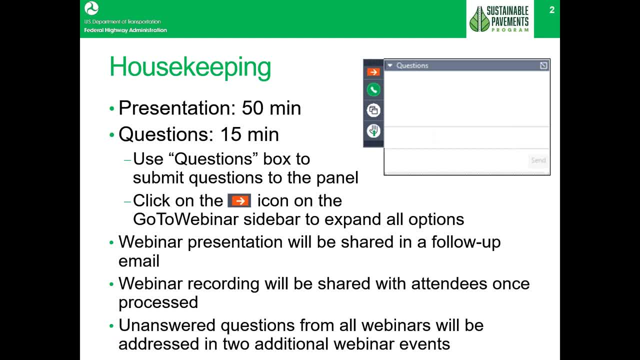 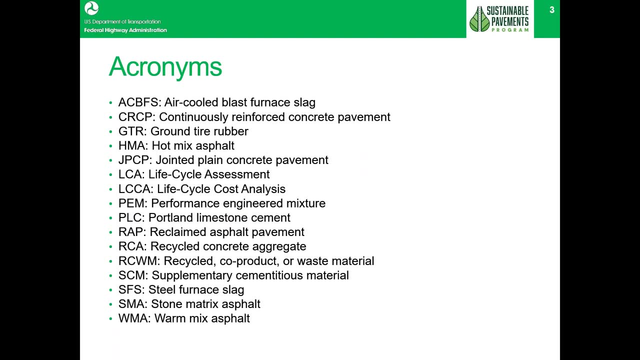 once it's processed. You may need to regularly monitor your spam or junk folders, as we found that some of our webinar communication occasionally gets redirected there. Throughout today's webinar, we will be using a number of acronyms referring to different materials, products and processes. We'll work to introduce these as they are used in 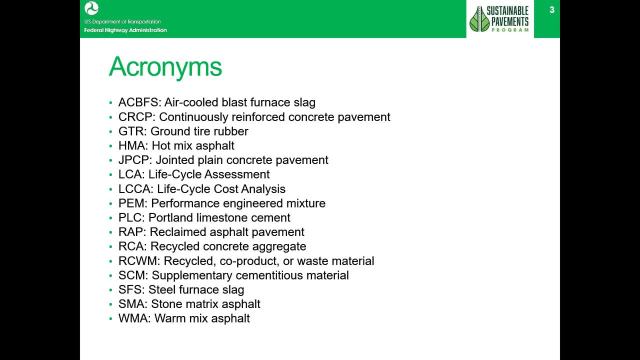 the slides throughout the webinar, but this master list will be available in the presentation that we share with everyone later. So now to get things started, I'd like to introduce Monica Llorado with FHWA, who will preface our webinar with a quick look at FHWA's 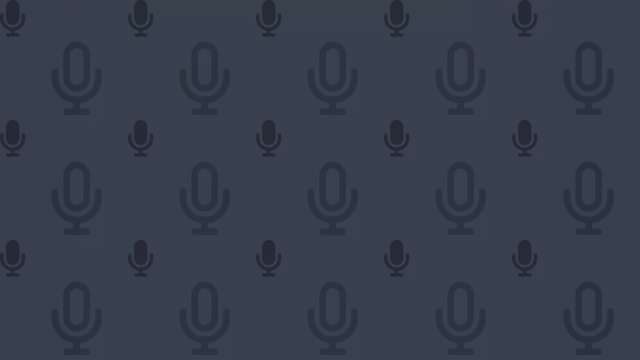 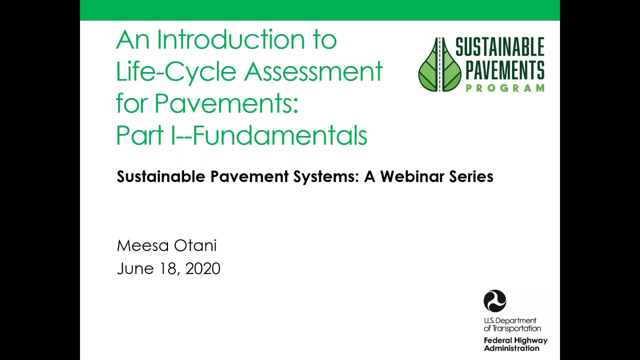 Sustainable Pavements Program- Monica. Yes, good morning to some of you and good afternoon. My name is Monica Llorado and I want to thank you for joining us for the Sustainable Pavement Systems webinar series and welcome you to our ninth webinar: an Introduction to Lifecycle Assessment for Pavements, Part. 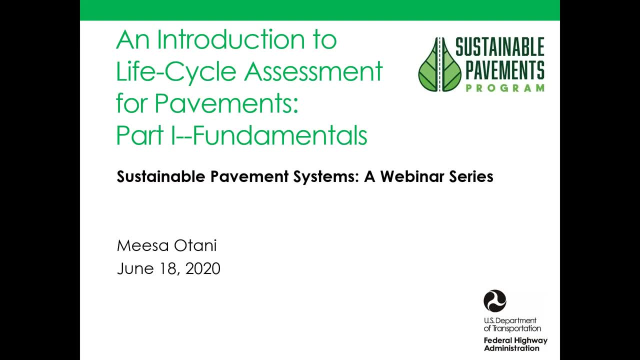 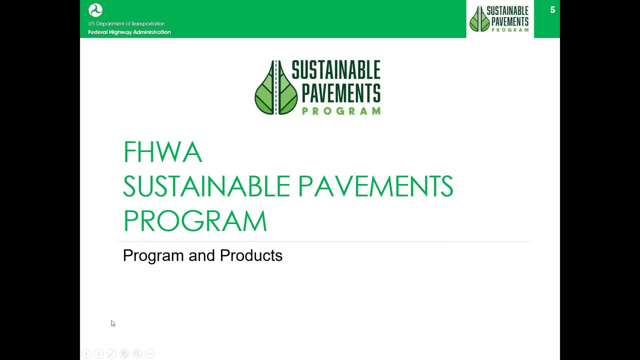 One Fundamentals. Before we get started, I would like to tell you a little bit about the Federal Highway Administration's Sustainable Pavements Program. So our program began in 2010 to advance the knowledge and practice of sustainability related to pavements, with the vision and mission. 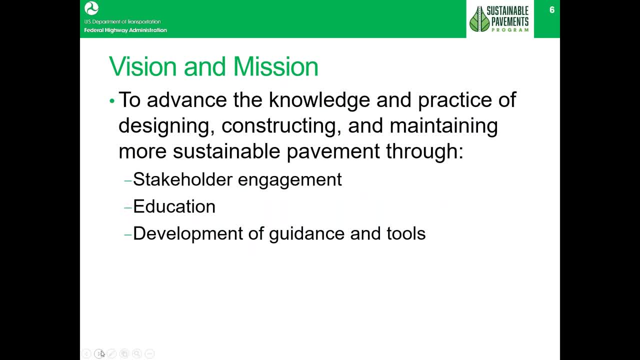 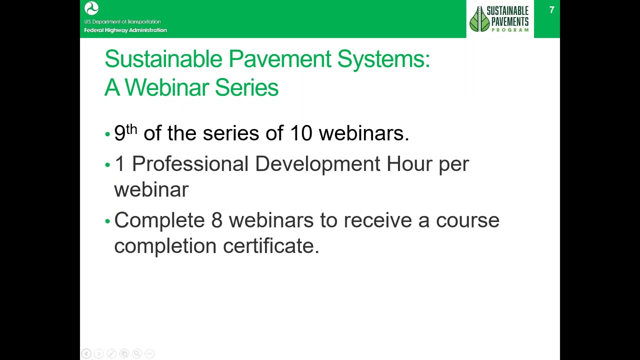 to advance the knowledge and practice of designing, constructing and maintaining more sustainable pavements through stakeholder engagement, education and the development of guidance tools, which this webinar series falls under our vision and mission. So, like I mentioned before, this is the ninth out of our series of ten webinars and you 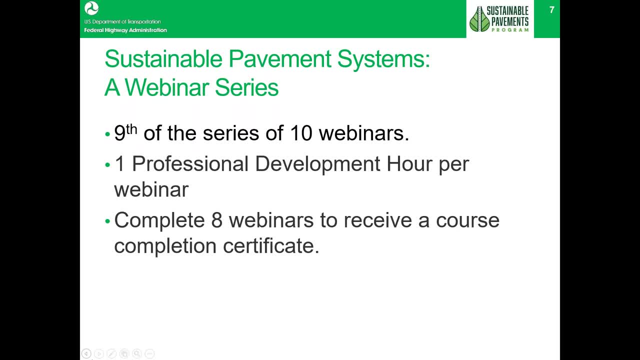 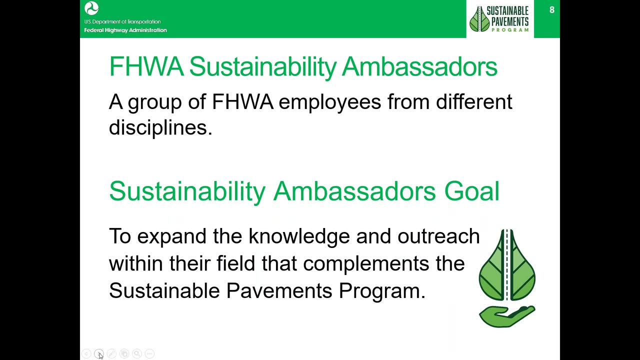 will receive one professional development hour per webinar and upon the completion of all eight webinars- eight out of the ten- you will receive a course completion certificate. Through our Sustainable Payments Program, we also developed the FHWA Sustainability Ambassadors, which is a group of FHWA employees from different disciplines whose goal is to 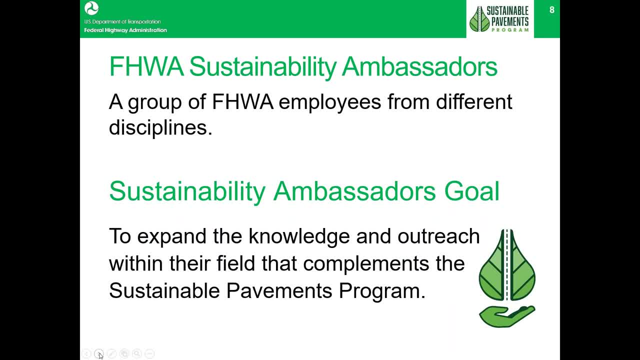 expand the knowledge and outreach within their field. that complements the Sustainable Payments Program And with that I would like to introduce our speaker for today, who is the Sustainability Ambassador, Ms Misa Otani, who joined Federal Highway in the Illinois Division Office through the Professional Development Program. 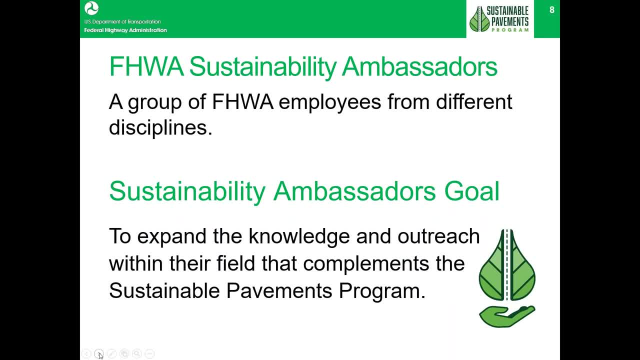 Following the PDP program, she served as the Environmental Coordinator for the Arizona Division from 2010 to 2012,. and in 2012,, Ms Otani moved to Hawaii, to the Hawaii Division, as the Environmental Engineer, which where she currently manages the Environmental Program. 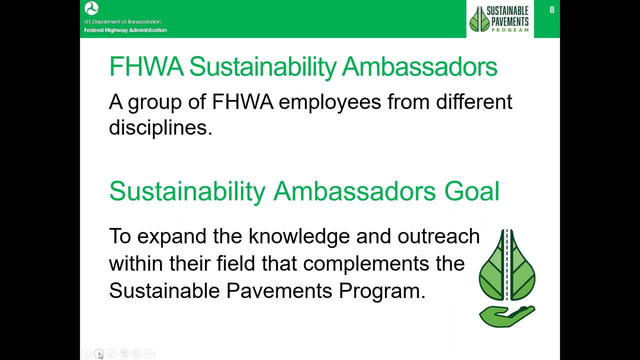 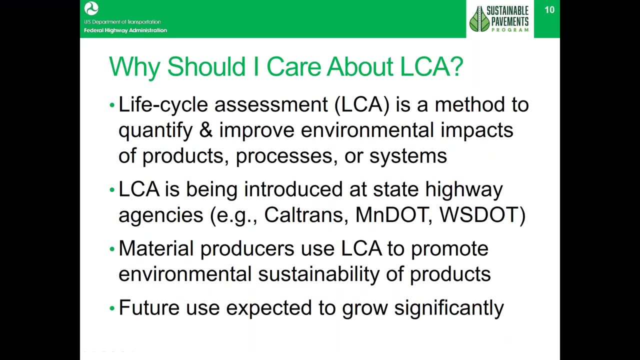 and serves as the Area Engineer for the Kauai District and the City and County of Honolulu. With that I'll pass on the microphone to Ms Misa Otani. Good morning everyone, or good afternoon to those of you on the East Coast. 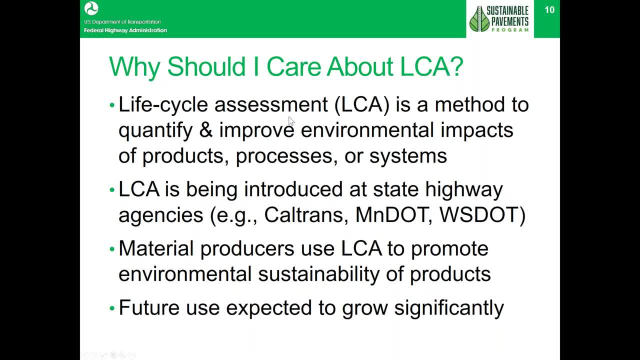 I'm Misa, as Monica said, and so I will be talking about life cycle assessment. So why should you care about LCA? Life cycle assessment is a method to quantify and improve environmental impacts of products, processes or systems. It's also being introduced at different state highway agencies, such as the Illinois Tollway. 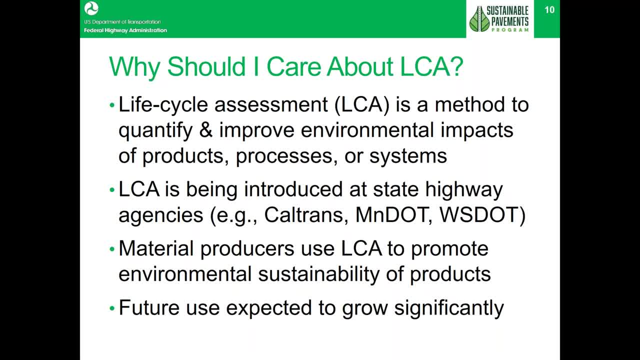 and the California Department of Transportation. Material producers also use LCA to promote environmental sustainability of products, and future use of LCA is expected to grow significantly. So the way the Illinois Tollway uses LCA tools is to evaluate environmental impacts of materials. 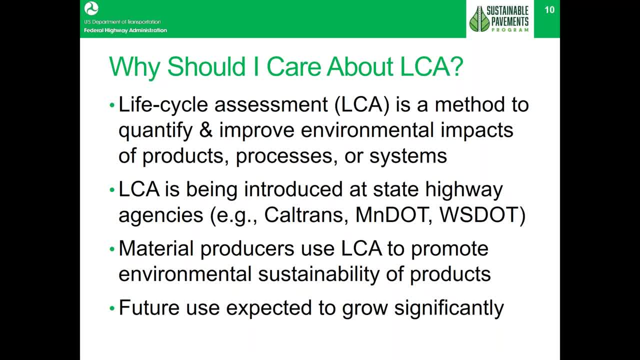 equipment and construction operations and uses that information in conjunction with life cycle cost analysis and sustainability rating systems in the decision-making process. The California Department of Transportation, or Caltrans, and the Oregon Department of Environmental Quality are also taking steps towards requiring environmental product declarations. 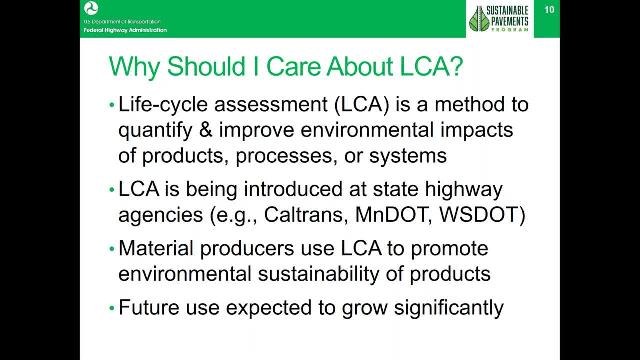 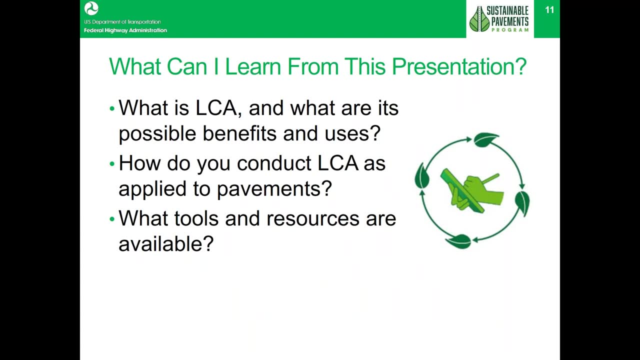 for pavement and other transportation infrastructure, materials for use in reporting, benchmarking and life cycle assessment for design and asset management, but not yet as part of procurement. Thank you, Thank you, Misa. Thank you, Thank you. So what can you learn from this presentation? 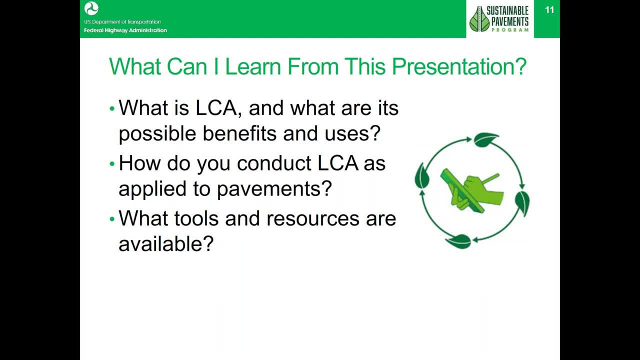 What is LCA and what are its possible benefits and uses? How do you conduct LCA as applied to pavements and what tools and resources are available? So, as I mentioned, life cycle assessment is an environmental assessment tool that is used by several agencies in the world, including the US. 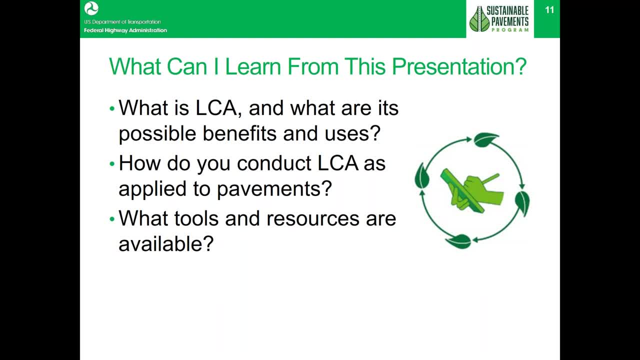 This presentation will provide you a short introduction to the current status of the use of LCA in the US and serves as a starting point for agencies and other stakeholders. In addition, it will provide you the opportunity to learn about the process, key issues and. 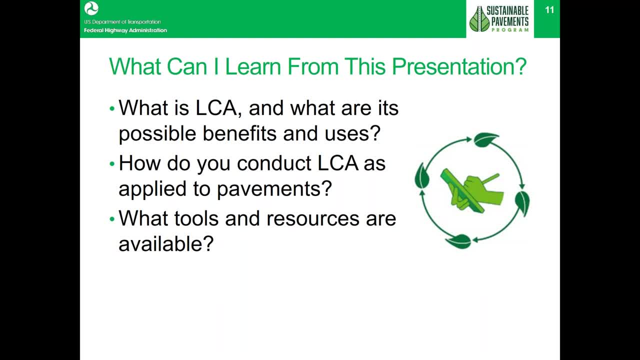 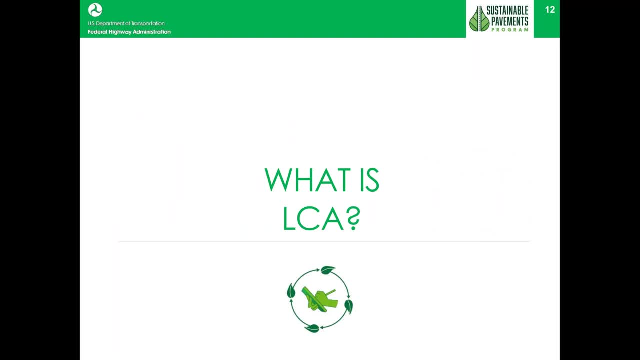 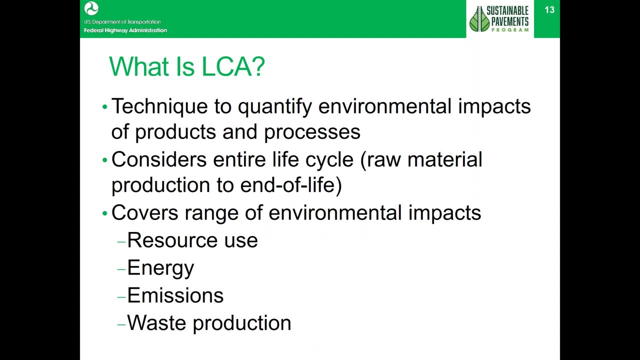 current applications of LCA for pavement. So again, we're going to talk about what is LCA. This section provides basic information on what it is. So what is LCA? It's a technique to quantify environmental impacts of products and processes. 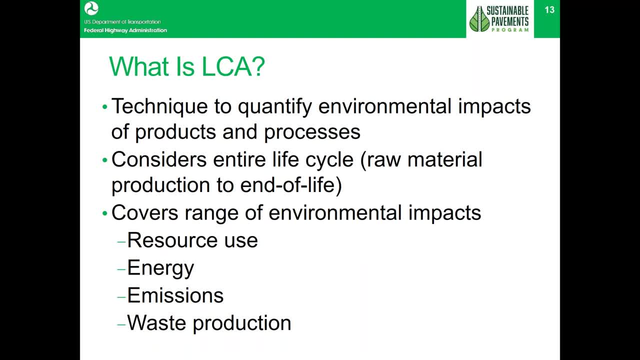 It considers the entire life cycle, from raw material production to energy sources, to environmental impacts of products and processes. It considers the entire life cycle from raw material production to energy production, end-of-life, and it covers a range of environmental impacts, including resource. 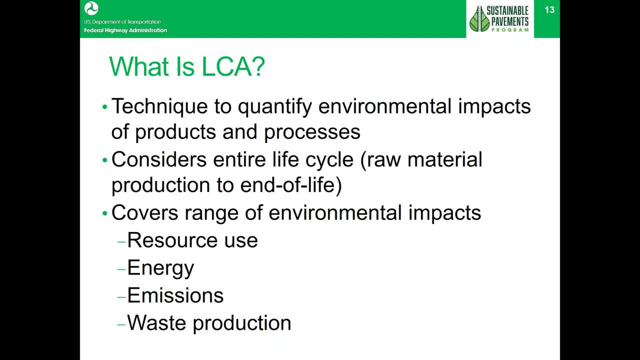 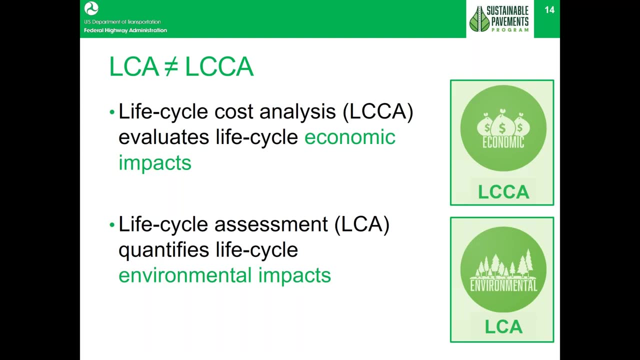 use, energy emissions and waste production. so LCA is a technique examines material and energy inputs and outputs over the entire lifecycle of the product or process and, as I mentioned earlier, lifecycle assessment is not the same as lifecycle cost analysis. lifecycle assessment quantifies lifecycle environmental impacts and lifecycle cost analysis evaluates. 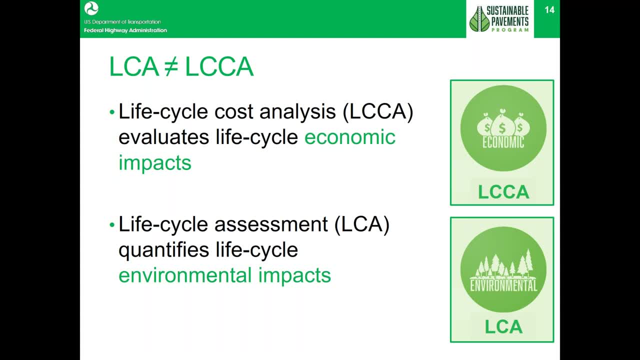 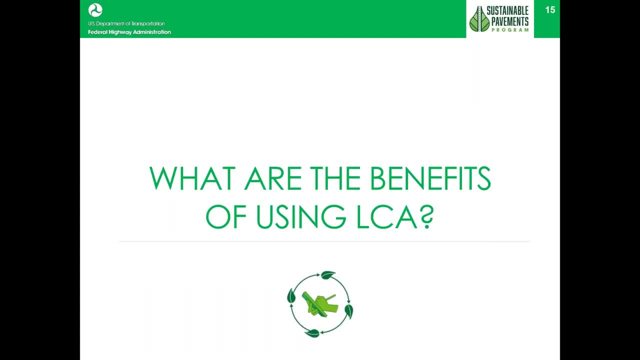 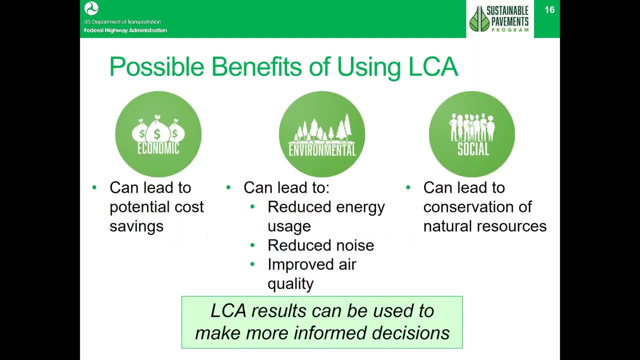 lifecycle economic impacts. so if you tuned into the last couple of webinars, it talked about LCCA. so the benefits of LCCA are going to be further discussed here. so a few examples highlighting the benefits of conducting an LCA to improve payment sustainability are shown on this slide. 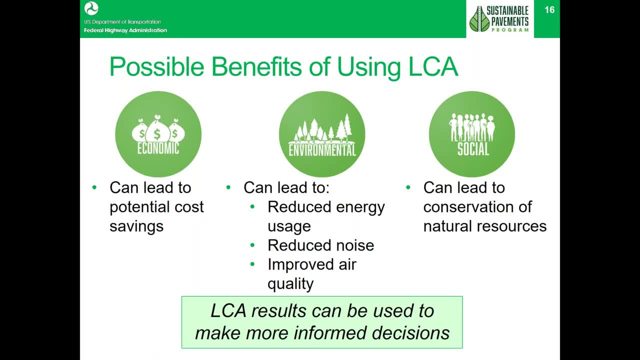 you so, where I talked about LCCA, can be used to improve the economic component of sustainability. the environmental aspect, which is LCA, can lead to reduced energy usage, reduce noise and improved air quality, and then also the social aspect can lead to conservation of natural resources. there is a unique opportunity. 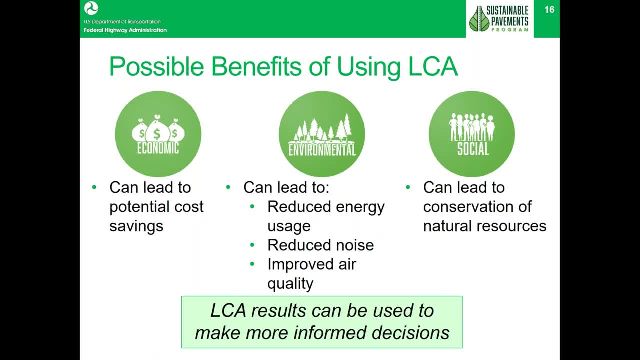 to improve the sustainability of payment structures, with the potential to deliver tremendous environmental, social and economic impacts, which, as mentioned in one of the earliest webinar series, is considered the triple bottom line. and with regard to those components, you know LCCA. LCA can be used to make informed decisions when you are going through a process. 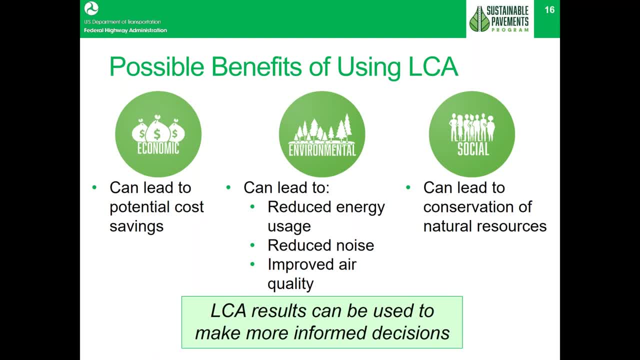 so these are some examples of metrics or priorities or values that may be considered in each of WSAC's Jenner Manual Templates heute. So if you take a picture of LCCA as a quantity, you know. so the two things down in this slide that I talked about. are really that significant everyone and again. also, you have to go out and get a some Jasmine Darkness in relation to these three parts here that I also like to complementary this秋, that I like to compare withmare trashen CEO or LCA- or LCA are important and you can track that behaviour and can make some decisions along the way, as you. northern airies are one of the most critical issues of theиса: abortion. 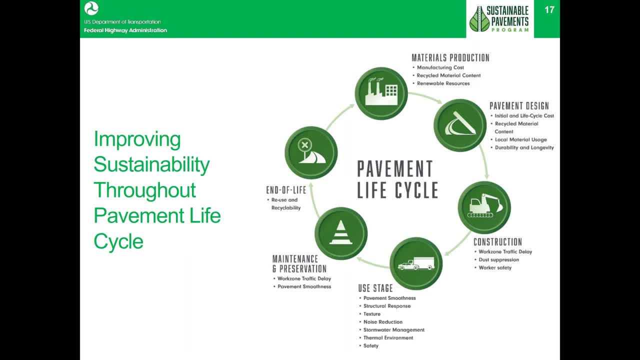 considered in each individual pavement lifecycle stage. So, for instance, for materials production, you might consider the manufacturing costs or recycled materials. In construction you're gonna think about worker safety or work zone traffic delay, And at end of life you're gonna think about reuse. 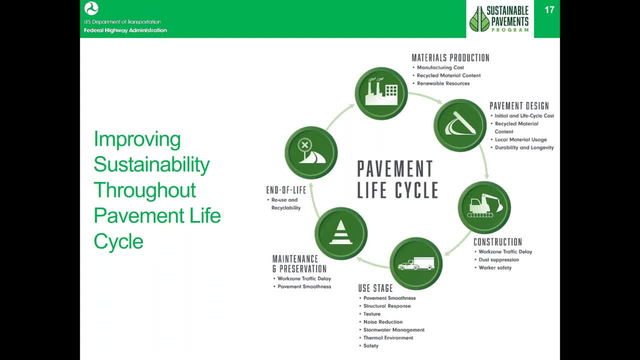 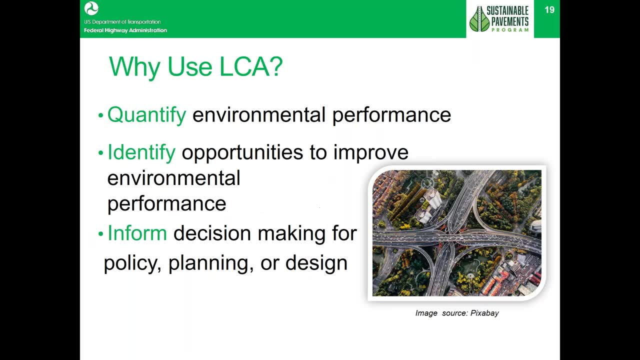 and recyclability. So how can LCA be used? First, why should you use LCA? It can be used to quantify the current environmental performance, which can be used to benchmark current practices and materials. With those current practices benchmarked, then you can identify opportunities. 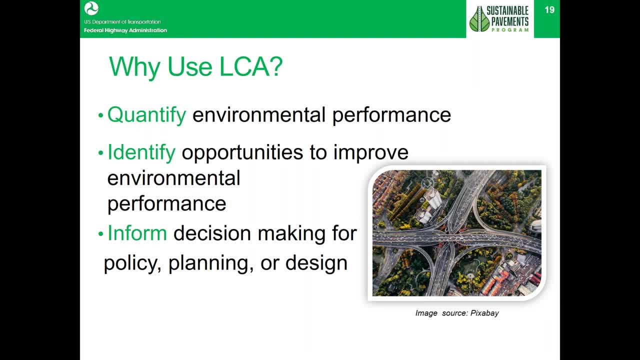 to improve the environmental performance which can be evaluated, measured and tracked to then help inform and guide decision-making at a number of levels which we will talk about in the next few slides. So for project-level applications, you can determine your pavement structural. 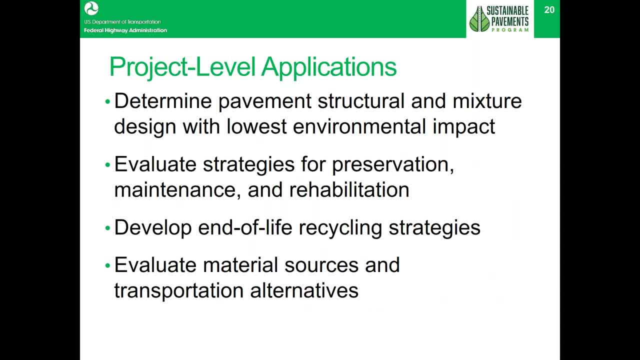 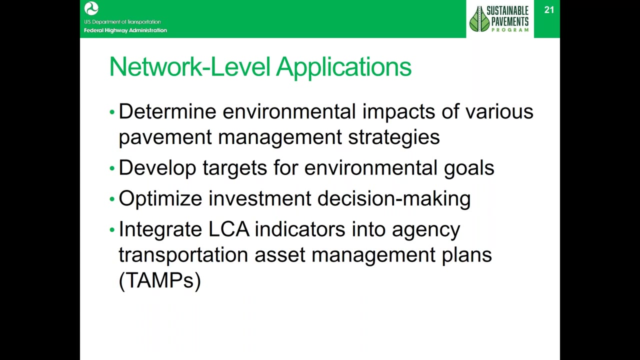 and mixture design with the lowest environmental impact, evaluate strategies for preservation, maintenance and rehabilitation, develop end-of-life recycling strategies and evaluate material sources and transportation alternatives. As part of a network-level application, you can determine environmental impacts of various pavement management strategies. 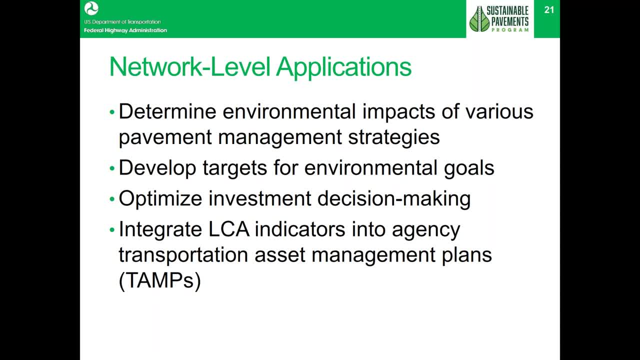 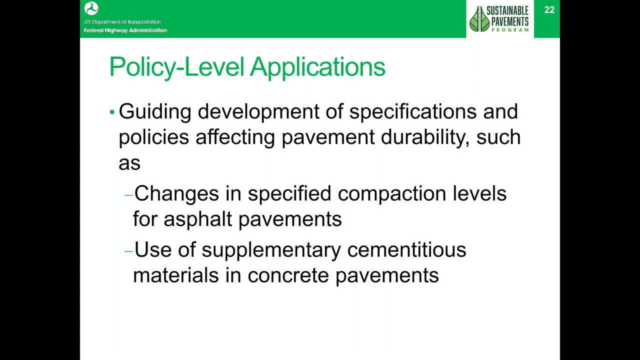 develop targets for environmental goals, optimize investment decision-making and integrate LCA indicators into agency transportation asset management plans, also known as TAMPs. And then, on the policy level, it can guide development of specifications and policies affecting pavement durability, such as: 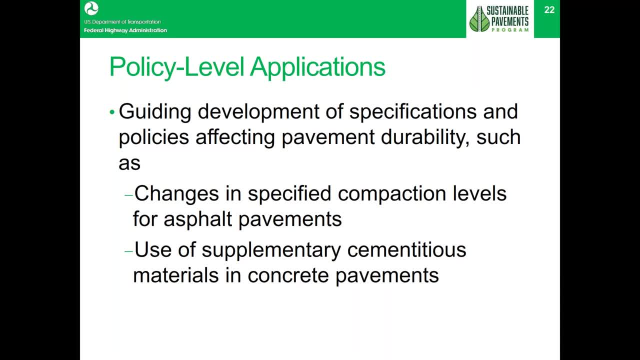 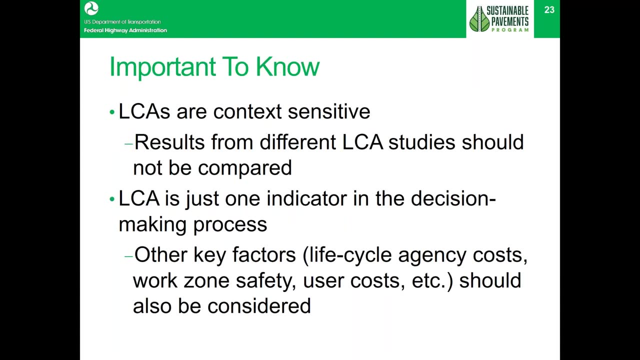 changes in your specified compaction levels for asphalt pavements or the use of supplementary supplementary cementitious materials in concrete pavements. So what's important to know? The results from different LCAs should not be compared because they are context-sensitive. LCAs to sorry, since LCAs perform to address. 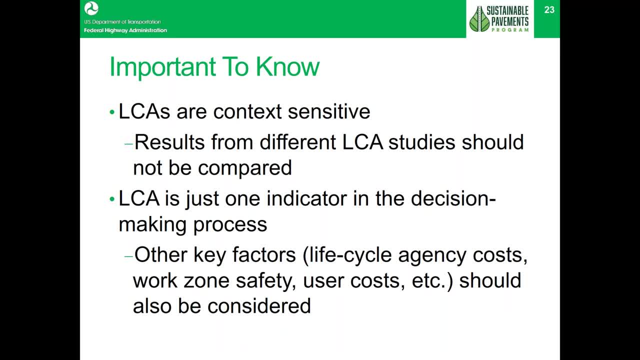 a specific question for a specific product or process that provides a specific function and a specific geographical location. So all of that just to say no results? no, true results from LCA studies should be compared, And LCA is also just one indicator in the decision-making process. 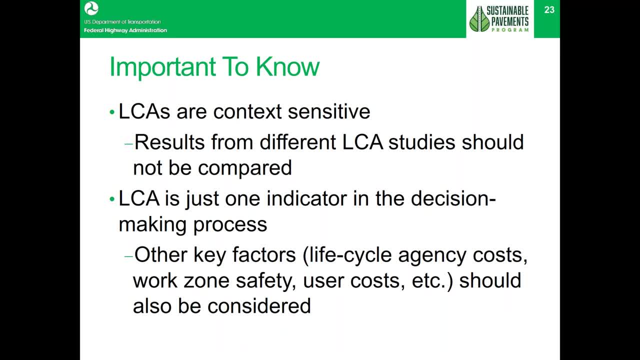 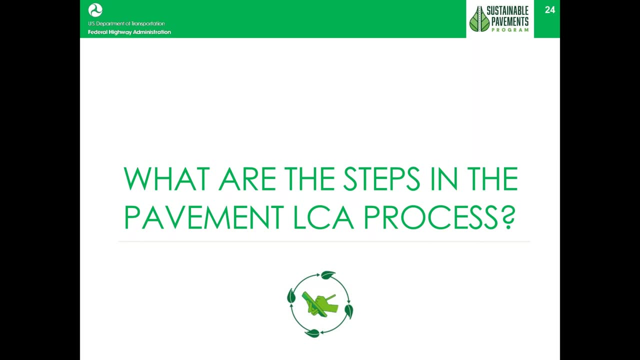 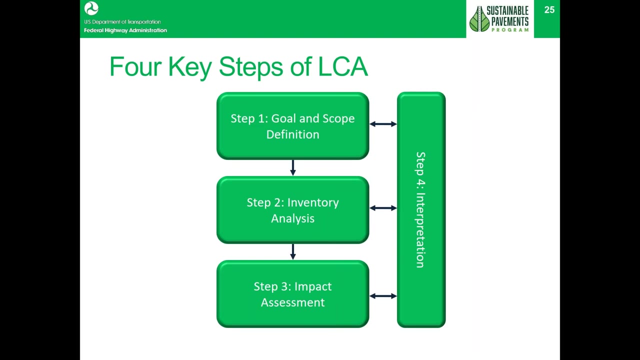 You have to consider other key factors, such as lifecycle agency costs, work zone safety, user costs, et cetera, in determining what you know, how you make your decisions as an agency. So what are the steps in the pavement lifecycle assessment process? There are four basic steps to the LCA process. 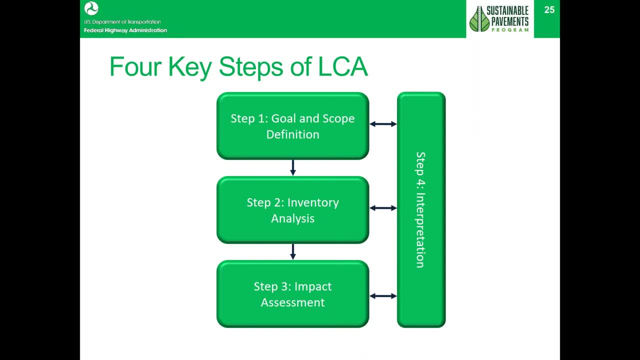 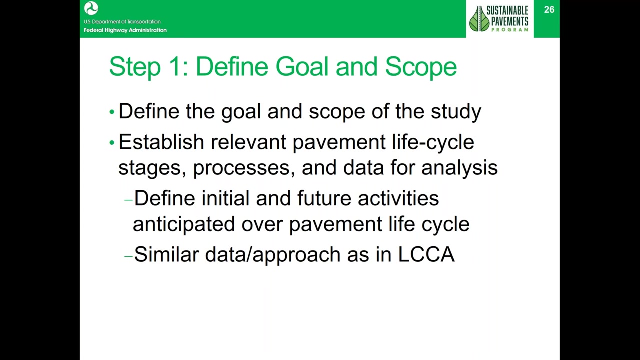 which are defined in the International Organization for Standardization, 14040 or ISO, which is the step one, is the goal and scope definition. step two is an inventory analysis, step three is the impact assessment and step four is interpretation. All right, so, for the first phase of an LCA, determines key features of the analysis. 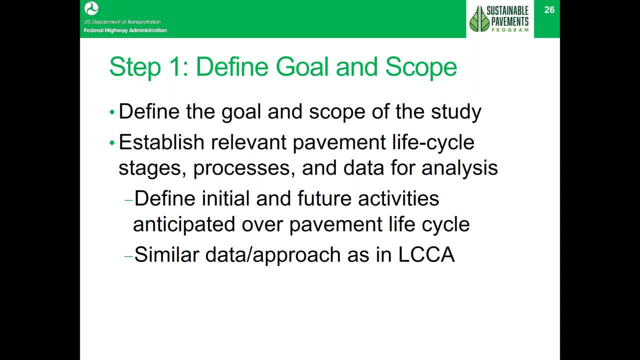 including the depth and breadth of an LCA, which can differ considerably depending on the overall goal. The scope of an LCA defines the system boundary of analysis. so basically, what's what life cycle stages and processes are included in the LCA? the geographic and temporal boundaries of analysis. the functional unit of analysis. 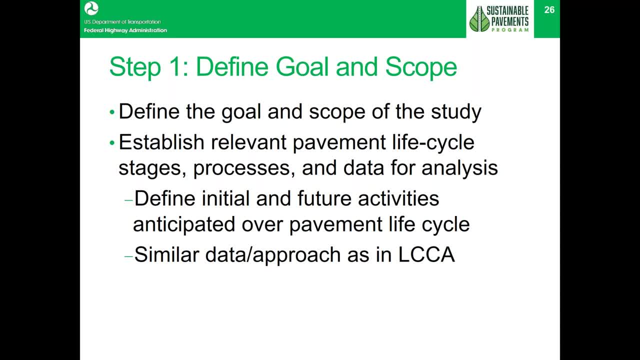 and also determines the required quality of data. Again, all of these depend on the subject and the intended use of the LCA. As an example, an agency may have the following LCA goal: To determine the environmental impacts of a pavement structural design. With that goal, 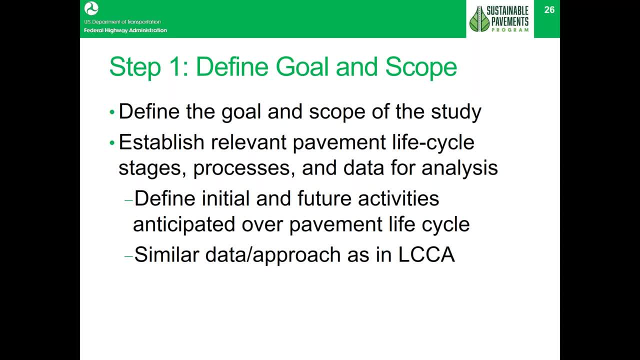 established. the scope needs to be defined with a partial list of some of the items to consider in developing the scope listed. Which life cycle phases are we going to include in this study? Is this going to be a cradle to gate study or will this be a cradle to grave study? 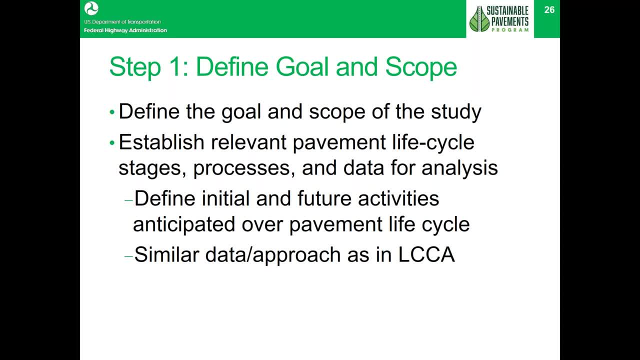 Are there some pavement life cycle stages that will be excluded? Will the LCA undergo a critical review? What are the system boundaries, What are the allocation rules being considered And how is certainty being handled? The key decisions made from this assessment are typically documented. 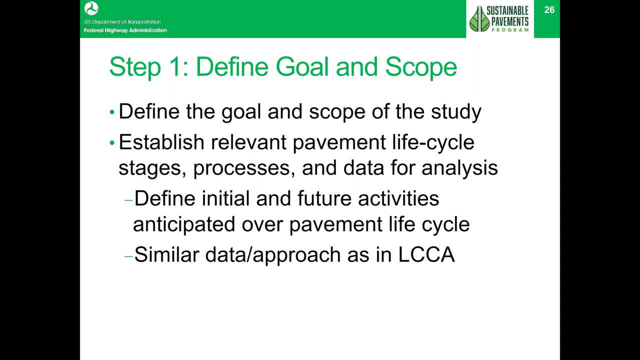 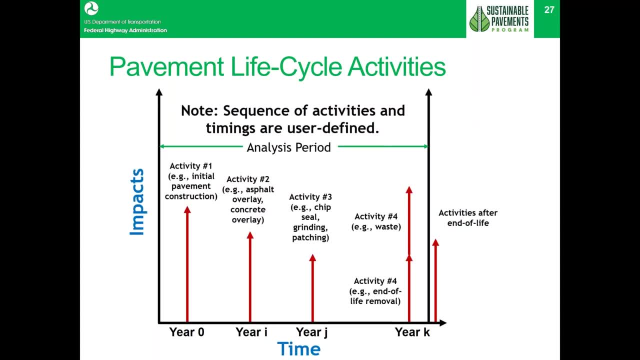 in a goal and scope document for the LCA being performed. So, as you can see on this slide, LCA's plot is similar to the life cycle cost analysis, where along the y-axis we would look at agency user costs and for LCA we are looking at environmental impacts. So this is just a brief. 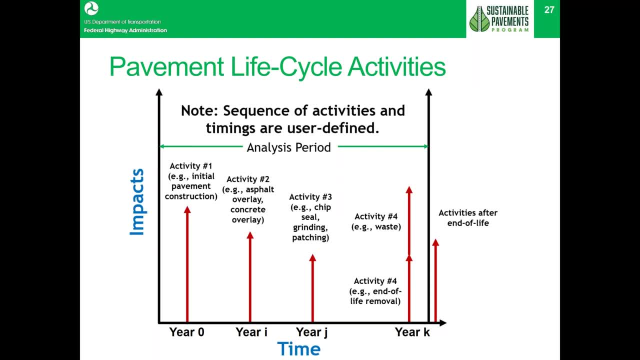 summary of what the local LCA can offer. I have given you a few examples of different activities to consider, such as initial pavement construction, or ask if you're going to do asphalt overlay or chip seal And then the end of life removal of that product. 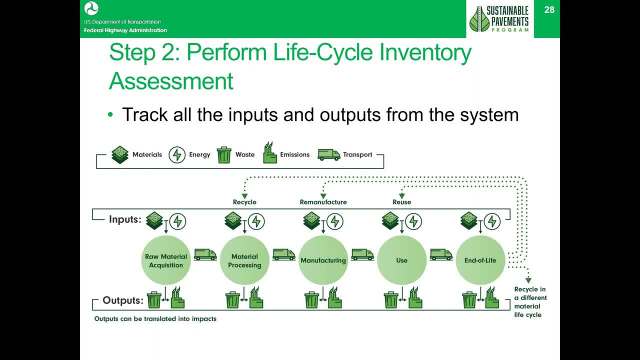 So step two in the LCA is to perform the life cycle inventory assessment, So you track all the inputs and outputs from the system. These input: these are inputs of resources And outputs of waste, estimated for each activity to produce this lifecycle inventory assessment. 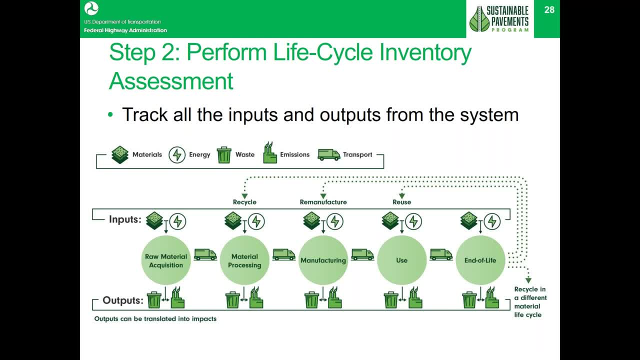 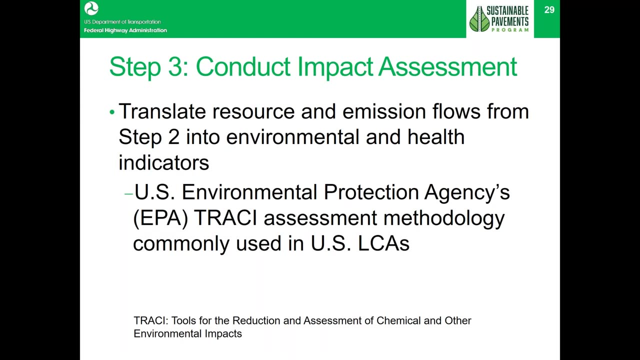 resource flows, considered our energy and materials, whereas emission flows are emissions to air, land and water. so step three of the LCA is to translate resource and emission flows from step two into environmental and health indicators: the resource, the resource and input and output flows, which can range from narrowly focusing on energy and greenhouse gas emissions to a 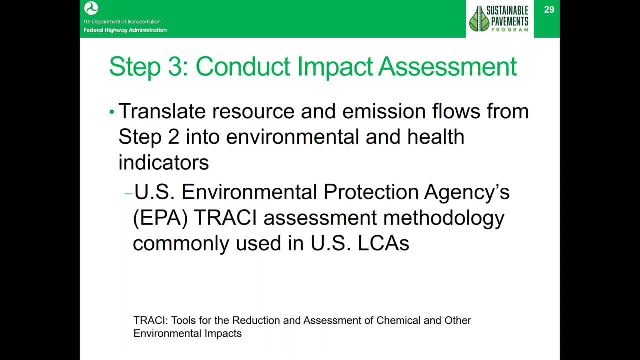 broader set of impact categories are translated into selected impact category results. the most commonly used impact categories in the US are based on the Tracy tool, or the tool for reduction and assessment of chemical and other environmental impacts. this is a tool developed by the US Environmental Protection Agency. 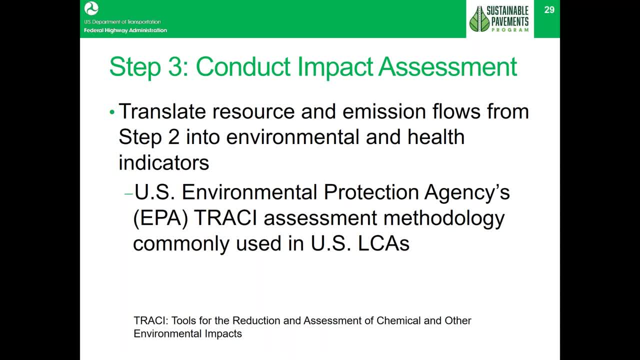 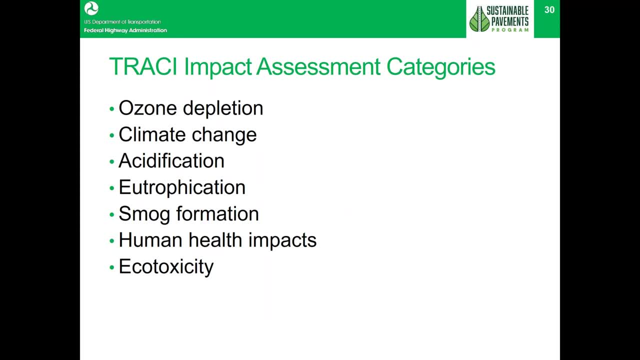 and on the next slide we'll talk about the impact assessment categories. so, as I stated, Tracy is an environmental impact assessment tool developed by US EPA. it provides characterization factors for lifecycle impact assessment, industrial ecology and sustainability metrics. characterization factors quantify the potential impacts that inputs and releases have on specific impact. 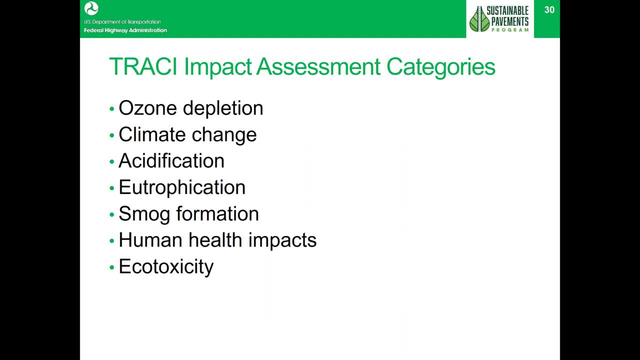 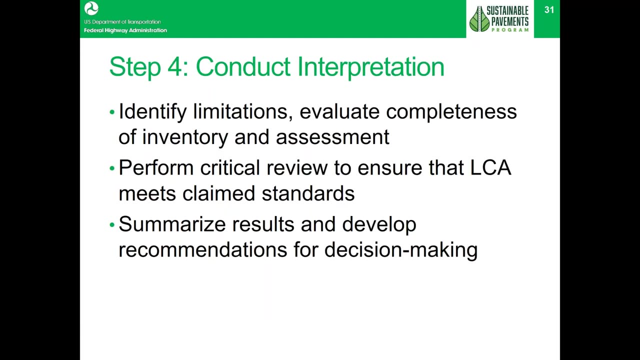 categories in common equivalence units. so, as you can see, the categories are: ozone depletion in climate change, acidification, eutrophication, smog formation, human health impacts and eco toxicity. so is the final step for an LCA. the overall results are summarized and recommendations are developed for. 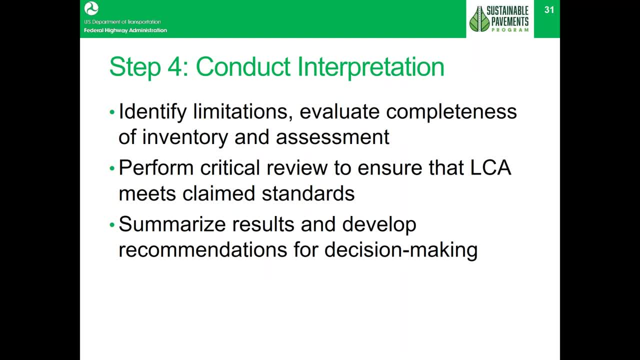 decision-making in accordance with the goal and scope definition. a review as part of steps one and for the LCA process by a carefully chosen grupo of experts, or stakeholders and providers that resolve questions- you'll see the or stakeholders- is recommended to ensure that the assessment meets the standards as claimed. 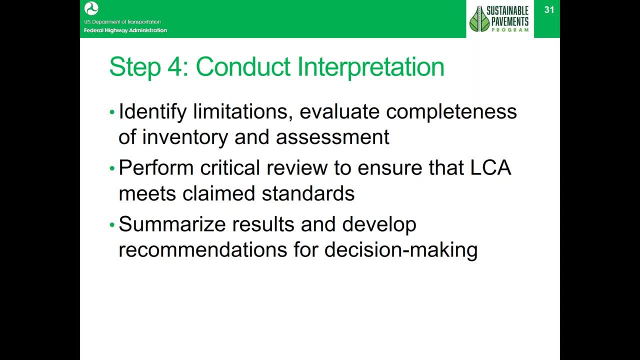 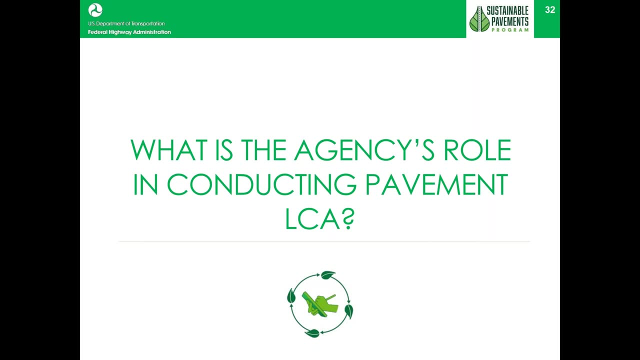 so, as part of this step, you'd identify your limitations, evaluate completeness of inventory and assessment, perform the critical review by a carefully chosen group of experts and stakeholders, and then summarize the results and develop recommendations for decision making. so what is the agency's role in conducting pavement life cycle assessment? 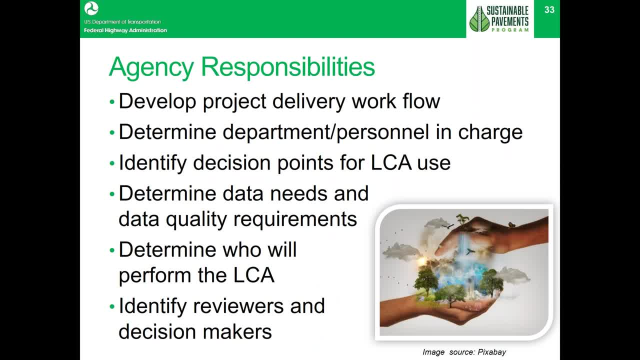 the different agency responsibilities include developing project delivery workflow, determining department or personnel in charge of lca, identifying decision points for lca use, determining data needs and data quality requirements, determining who will perform the lca and then identifying reviewers and decision makers. an agency needs to be actively. 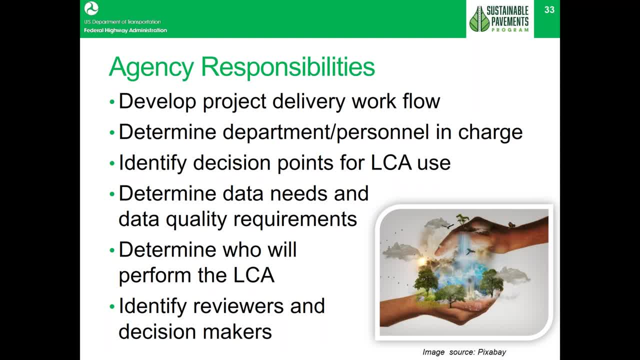 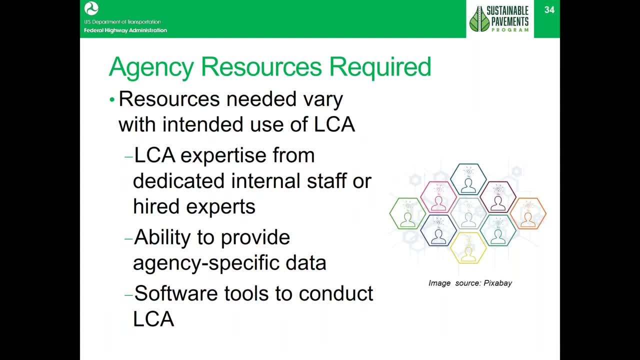 engaged in the lca process to ensure that it is relevant to the agency. so what are the resources required for an agency to use lca? resources needed vary with the use of how the agency is going to use lca, but they typically rely on the use of. 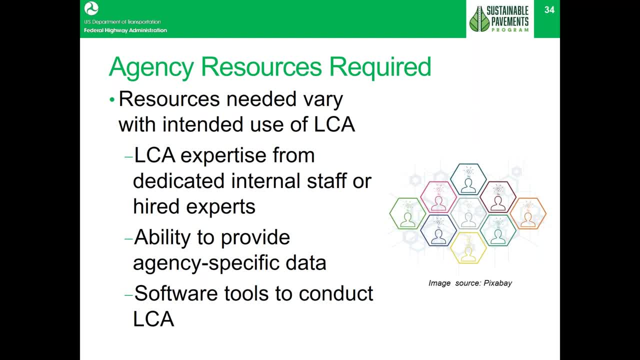 lca expertise from the dedicated internal staff or hired experts. there are a number of commercially available lca software tools and also spreadsheet based tools that include life cycle inventory data sets for pavement that can be used as a starting point to develop lca models, and some state agencies, some state highway agencies, have developed. 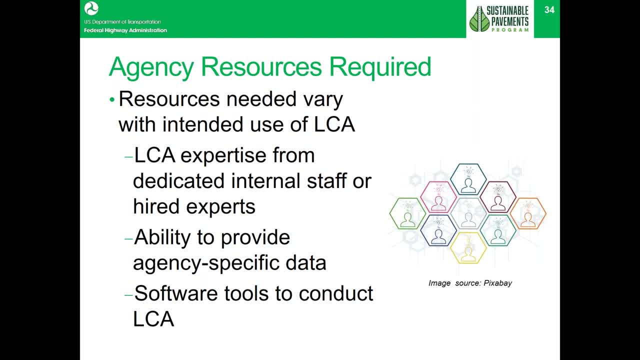 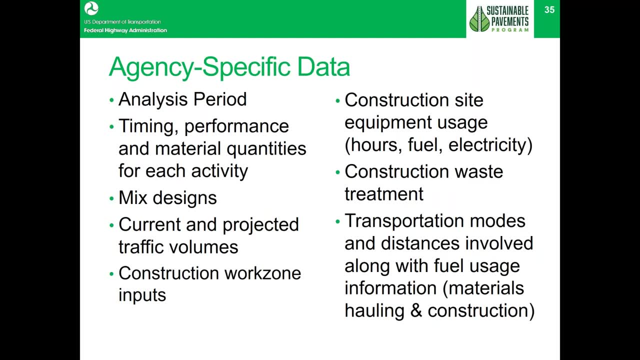 their own customized lca software tools with agency specific default background data. so some agency specific data that you would need include the analysis period, the timing, performance and material qualities for each activity, mixed designs, current and projected traffic volumes, construction work zone inputs, construction site equipment usage, such as hours, fuel and electricity, construction waste treatment, transportation modes and 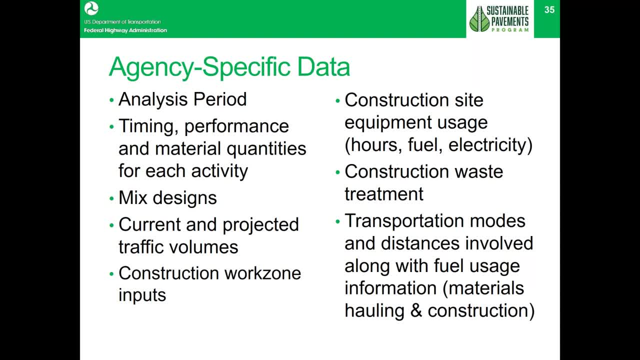 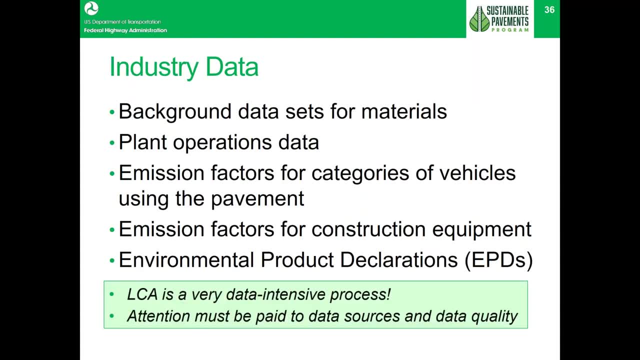 distances involved, along with fuel usage information such as materials, hauling and construction, and then industry data. you need a background data set for materials, plant operations, data, emission factors for categories of vehicles using the pavement, environmental factors for construction equipment or emission factors for construction equipment, and and also environmental product declarations. 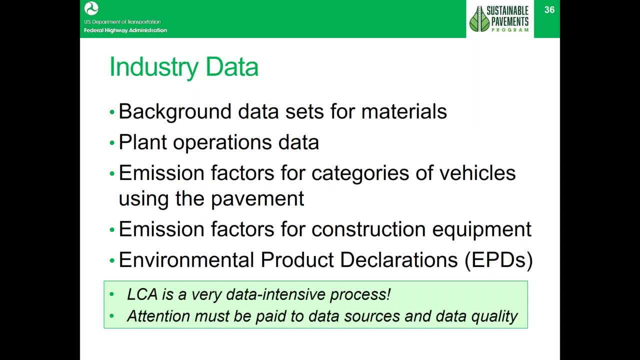 lca is a very data intensive process, so that's also something that everyone should be aware of, and attention must be paid to data sources and data quality, because, basically, if you're going to put something that's not quality data in, you're not going to get quality data out. 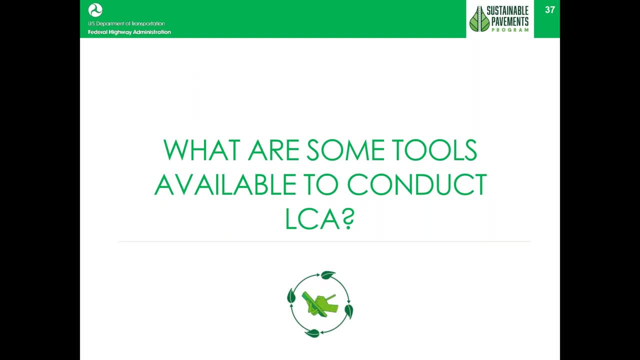 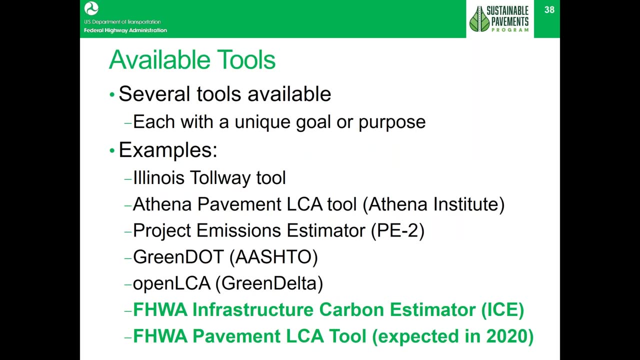 so what are some tools available to conduct lca? okay, I think now's the best time of the year to discuss it. staff resources related to ええ is good to be in the know to get the benefits of yourобр fulfishing. that's something you should. 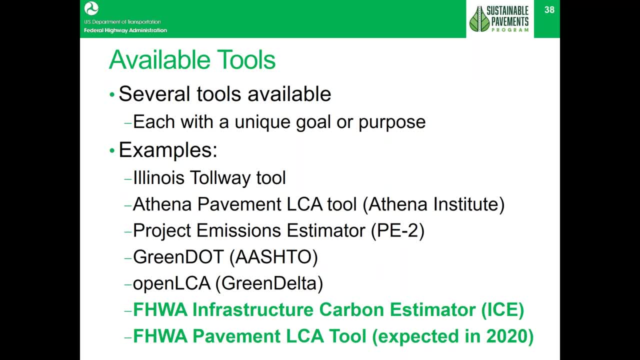 be laying back and consider though, and maybe it's a little bit of a crit issue, but thank you so much for reminding me to focus more on the democratizing 음악 group right now. and also, I really think these insights are scary planning strategies, as you're learning. 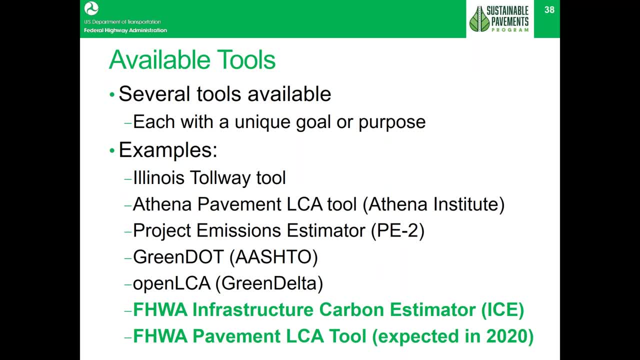 because in the broader publica- and I'm talking more about national pw now, but you might be able to Påry- it's not in a module where anyone can answer- is my question. I would just like to use your experience, but but you've obviously had some questions that you want to answer. so if you have a message or 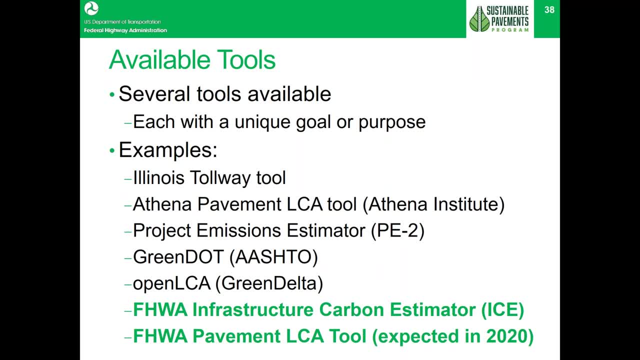 please keep it within that chat box, a short one, and please lower your figures. if you have a question or comment, please, if you want to start a discussion, if you want to show, if there's anything you want to talk about, please, going to be presented in a webinar, hopefully this summer, so look out for. 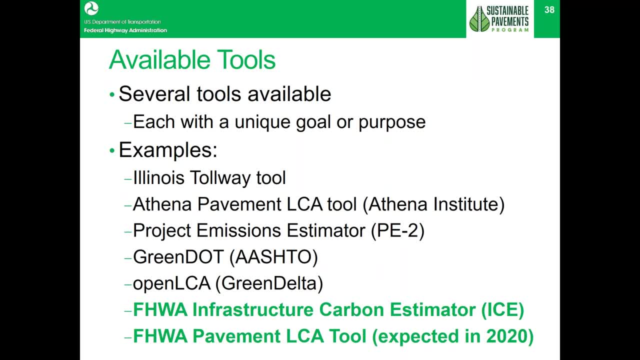 updates on that, and then also the federal highway pavement LCA tool, which is currently being developed in accordance with the pavement LCA framework that was prepared in 2016, and FHWA's pavement LCA tool is being developed with input from state highway agencies, with the pavement industry in. 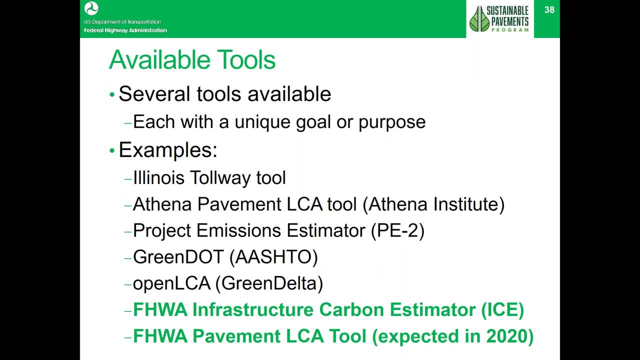 addition, a dedicated group of potential users from state highway agencies, which is the pavement lifecycle thinking task group, are also guiding the development of the tool. this group is closely involved in all stages of the development of the tool and it will make use of public and open source data sets. 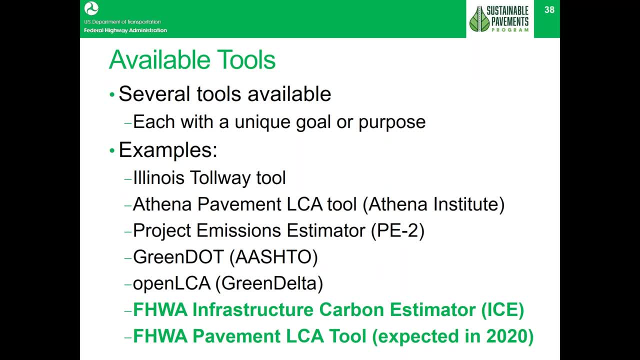 so talking about some of the other tools, the Illinois tollway through tool includes pavement structures, drainage, lighting and landscaping. the PE tool tool includes greenhouse gas emissions models for construction maintenance and use, and Green Dot from Ash Topher performs a high-level carbon dioxide calculation from the operations. 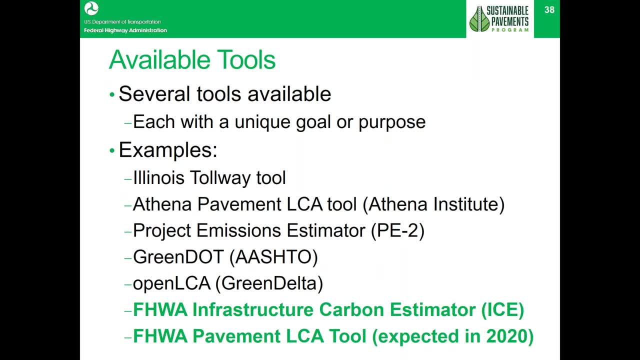 construction and maintenance activities of state highway agencies, and the open LCA is an open source LCA tool. it is being used by the federal LCA Commons, which you can find out more about at wwwlcacommonsgov. so where can I find more information? 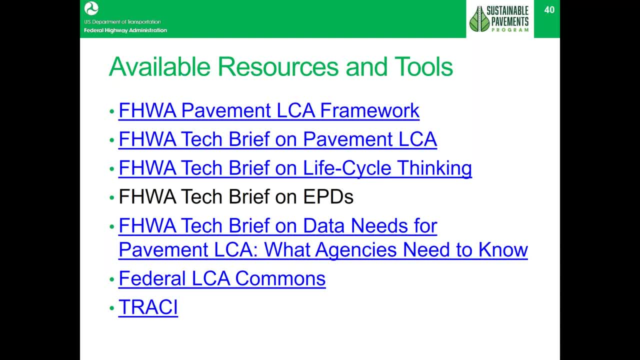 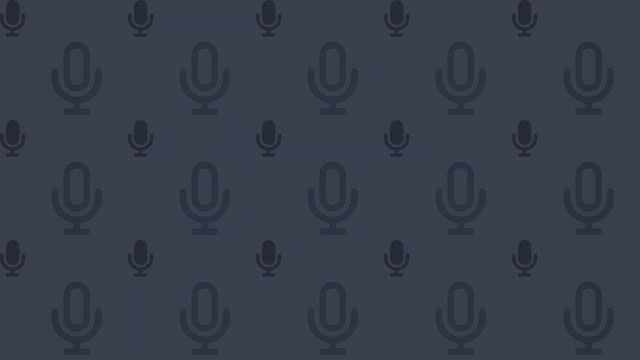 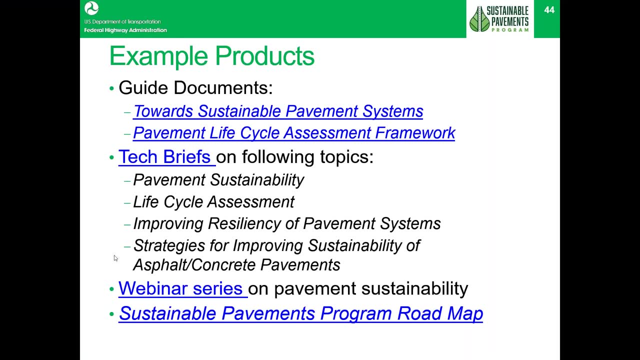 and I think I turn it back over to Monica. yes, so some of the products that we have in regards to with the sustainable payments program includes our towards sustainable reference documents. we also have a LCA framework document and all this information can be found in the LCA. 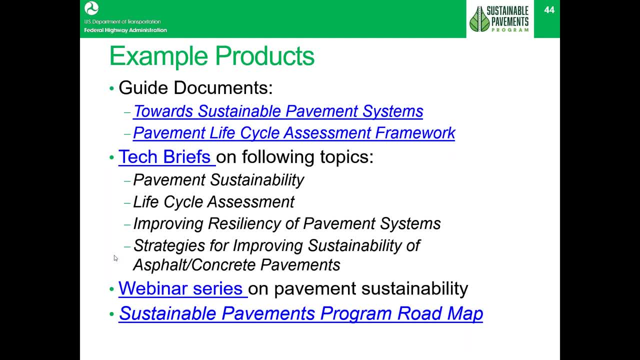 and all this information can be found in our website, which also includes some webinars, technical briefs that we have, such as technical briefs and payment sustainability lifecycle assessment- and others in improving resiliency of pavements. and the most important, or what we call one of our most important. 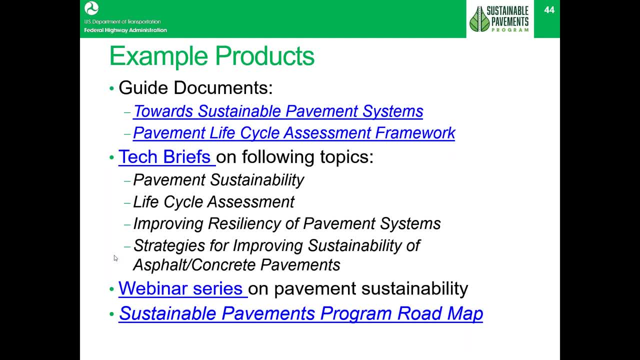 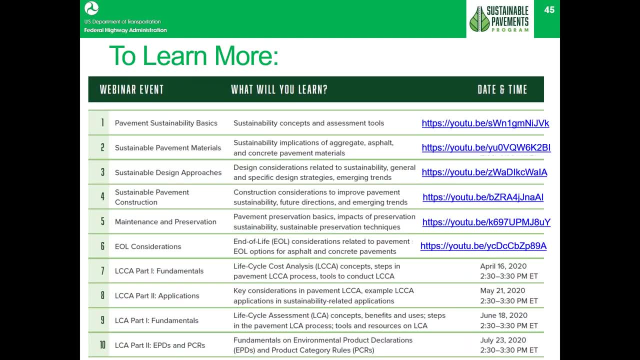 documents is a sustainable payments program roadmap. on the next slide we'll be able to see the links to the recorded webinars which you have been receiving through emails if you participated or requested or registered for the webinar, and we would like to enjoy, invite you to our last webinar, webinar number ten, which is LCA part two, which is: 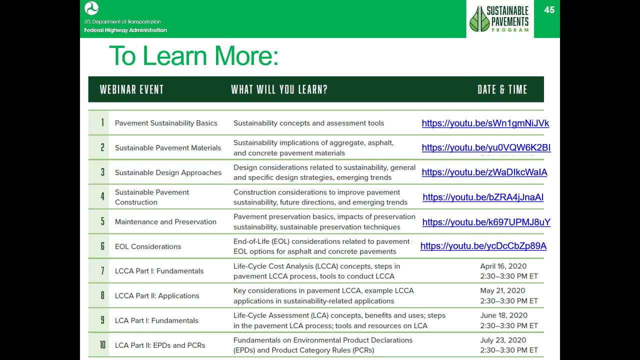 focused on EPDs and PPRs. EPDs are environmental product declarations, and that's the most important thing that we have to remember about the actual lives of renewable energy services in the. And PCRs are product category rules, and that will be July 23rd. 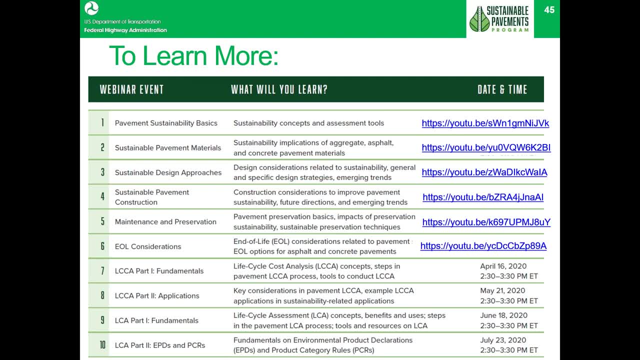 If you haven't signed up for it, please do so, And we are adding two more webinars. We're still in the scheduling process for – and it will be webinar 11 and 12, and it will focus on all the questions and answers that we did not get to answer throughout the 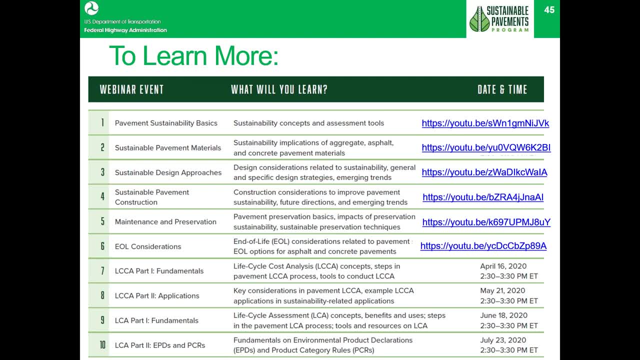 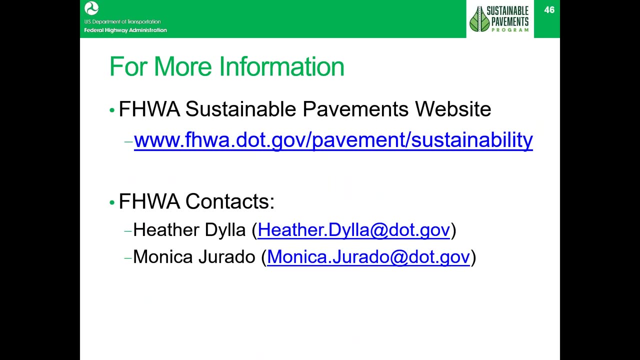 webinar series for all webinars 1 through 10.. And so we'll have those available too for you to register. And with that, if you have any questions, please feel free to contact Heather Dilla or myself, and also feel free to visit our Sustainable Payments website at any time. 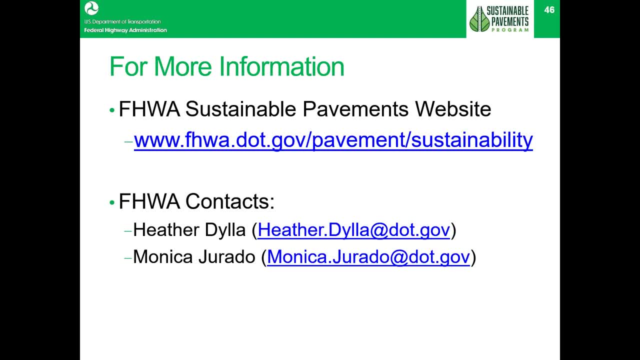 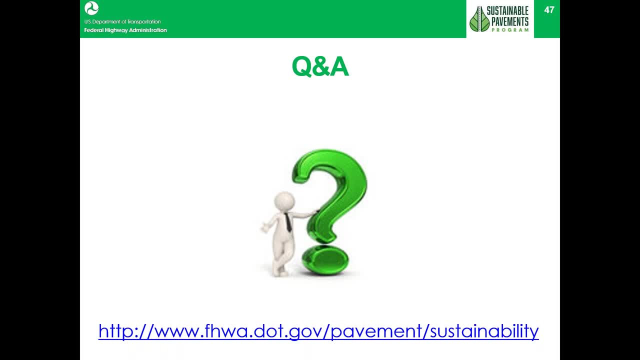 And with that I'll hand it over back to Kirk for questions and answers. Hi, Thank you, Monica, and thank you, Misa. We appreciate that overview. Again, remember that this is the first part of a two-part presentation on LCA, so we'll 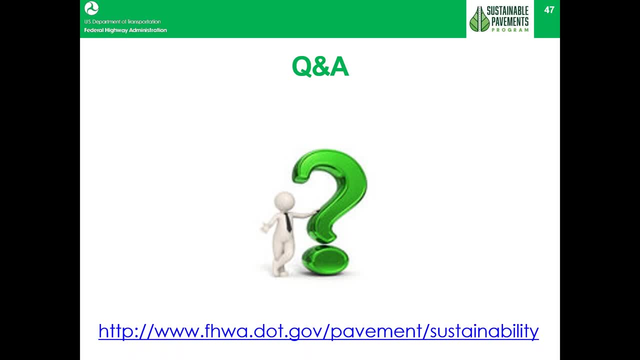 be following up again in a month on the second part. So this presentation was intended to kind of be an overview and kind of give everyone a flavor for what's involved with LCA. We've been receiving a few questions, but I would encourage everyone to submit additional. 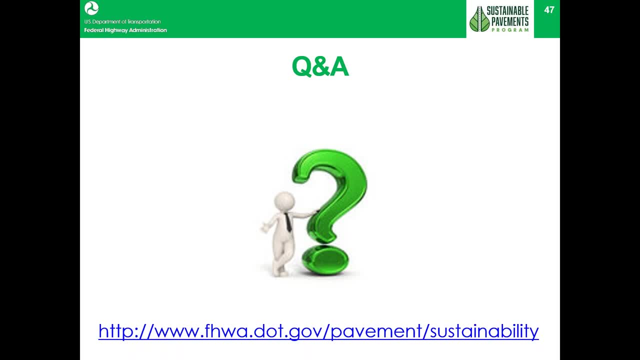 questions. If anything came up as we were going through the presentation material, Feel free to use the question box and submit some additional questions, Maybe just to get things started. we've got a couple here, Misa, I'll direct this to you. 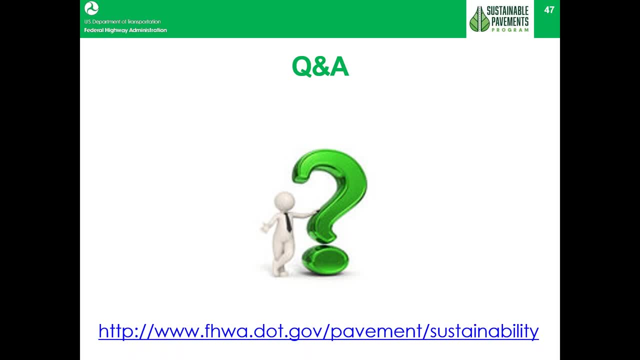 Question is: what are the most common environmental impact indicators and which ones are considered to be the most important? I think I'll turn that over to Heather. Okay, Sure, That's fine. Okay, So with regards to the impact indicators from the federal highway standpoint, we don't. 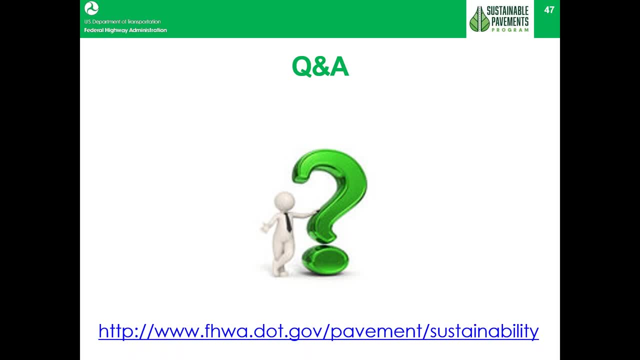 give any technical guidance on which is the most important. So I just wanted to clarify that That's really left to the states. But from what we are seeing as far as trends in the states that are either showing interest in LCA or have regulations that they're using LCA to help meet the current state regs, it 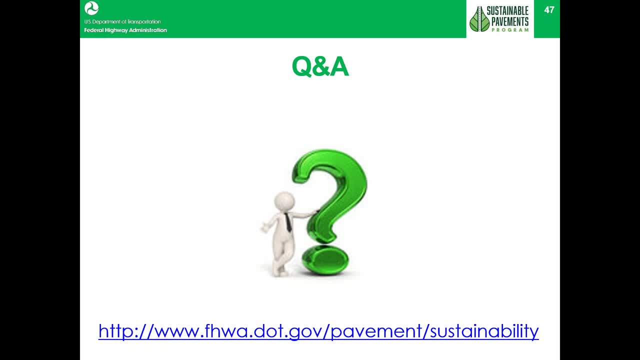 is usually focused on the greenhouse gas or climate change impact category or energy use. Those two are the ones that tend to be commonly used And it's the best practices to include all the impact categories. Tracy has numerous impact categories that Misa went over, such as acidification, eutrophication. 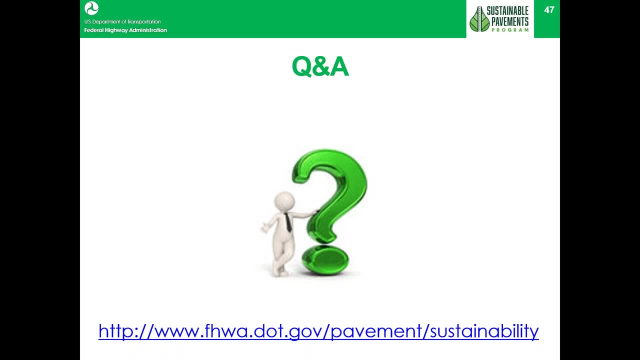 smog, ozone depletion, et cetera. And, of course, the other thing that was really helpful- and this was also on the table, but particularly around carbon emissions in the state- is that the best practices are to include the carbon footprinting and the carbon footprinting of carbon emission. 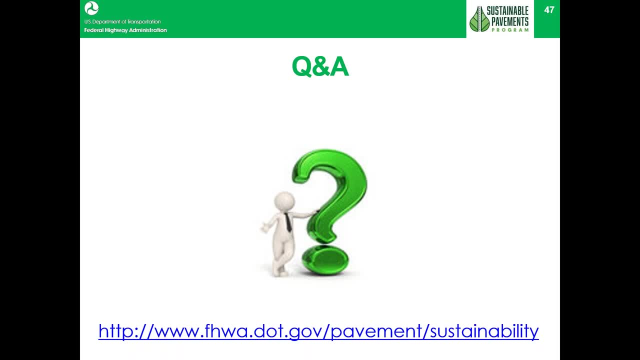 And I think that's a really important point Because there could be tradeoffs amongst them And so if you do just focus on one indicator, you could be missing some of the tradeoffs in the other indicators and not getting the whole picture. And, in addition, when you do focus on just climate change, it would actually be considered. 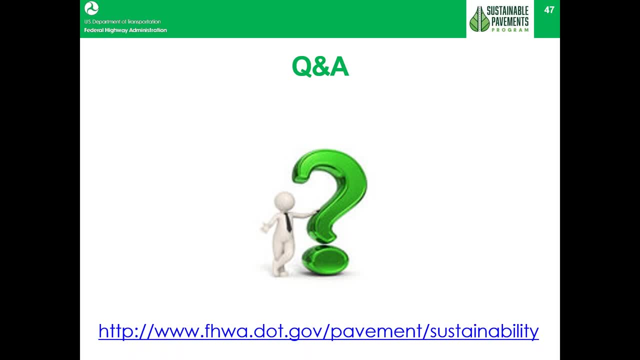 really is encouraging looking at all the different indicators, potential indicators. All right, Thank you, Heather, And I think Heather made an important point that it really depends on the agency or the user in terms of what may be most critical for them, depending on whether 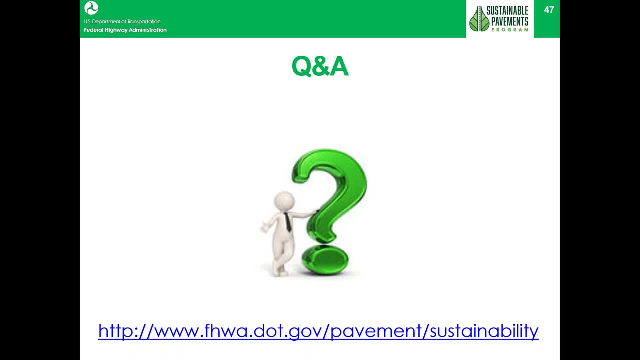 they have certain goals that they're trying to achieve, may dictate which of those different indicators might be the ones that they would be giving most weight to. Let's move on to another question, and I think I'll direct this one to Heather as well. 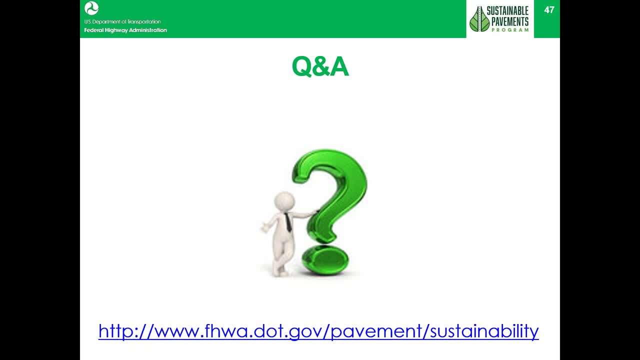 Heather. the question is: what is FHWA's view of product LCI, slash, LCA information from industry associations, for example Asphalt Institute or Euro Batum? That's a good question. So there was a slide that mentioned various tools and there are various tools out there and many of 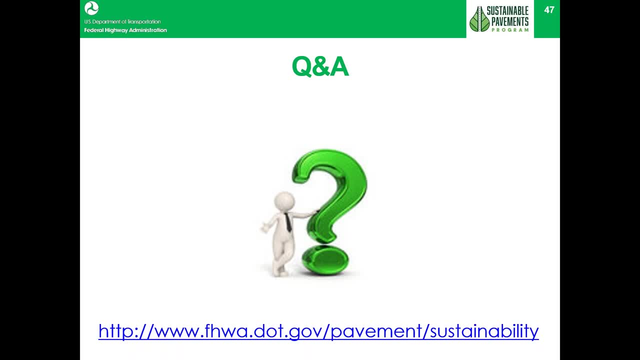 them have different data sources, And I think what's unique to the tool that is being created under FHWA is we are really trying to work with industry. what would be the best data that represents their industry? But then we're also trying to encourage harmonization amongst the 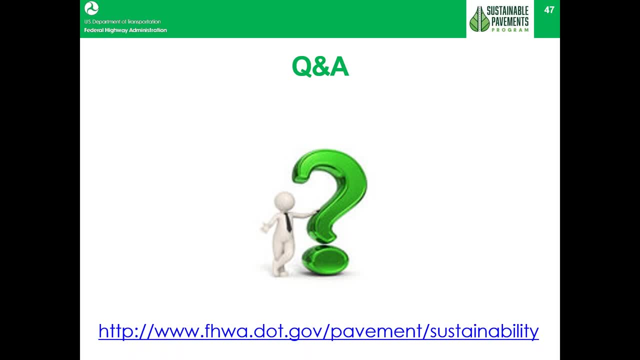 industries in what would be considered some of the background data sets that they use, or common background data sets such as electricity usage, et cetera. So we recognize that there is not harmonization in the approaches that's being used for these studies, but we're trying to encourage harmonization and we certainly want 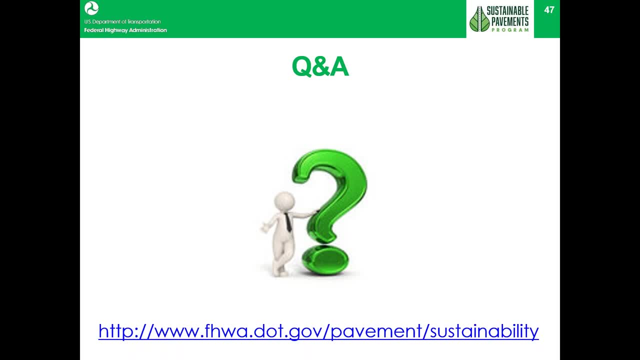 to work with industry on getting what is the best data into that tool. So some of those conversations, particularly to what was mentioned here- Asphalt Institute data or Euro Batum, the commercial databases- we're going to be having those discussions With regards to commercial databases. 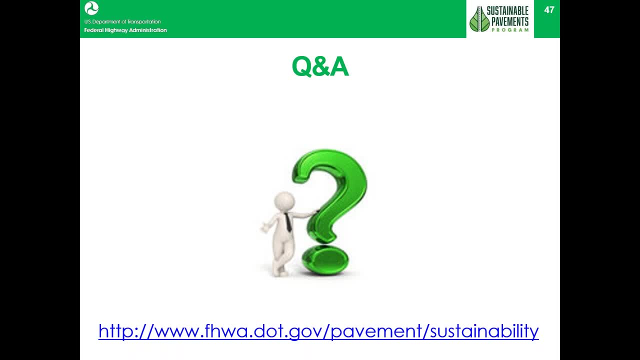 we believe it should be more. the data in the tool should be public data so freely available that anyone could access, And so therefore we're not putting in commercial databases per se. but, if you know, the data is in the federal commons. Musa mentioned the federal commons. it's where all 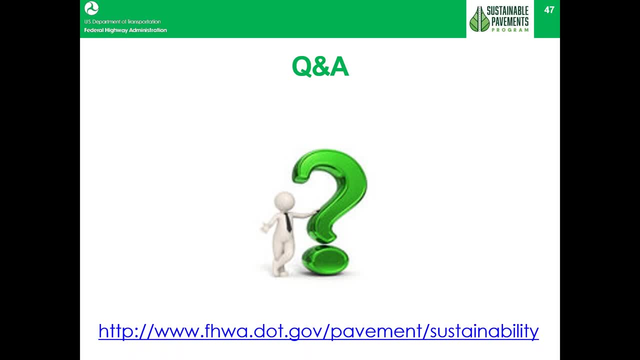 the US federal government data or some of the industry data that is provided to the LCI database is being published. So we would be largely encouraging industry to publish their data in the commons and then easily incorporating into the tool or work with industry to get it up. 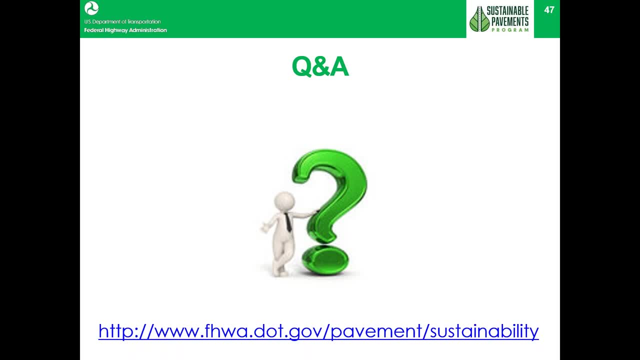 in the commons, et cetera, to make it more available and easily available. So we're going to be implementing it into some of the frameworks and ongoing efforts we have, So that, I think, pretty much covers it With regards to 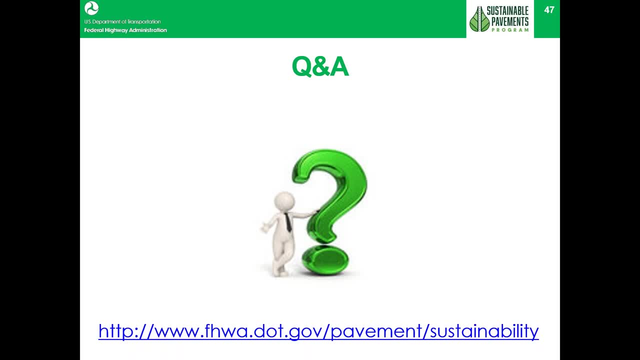 some of the reliability and certainty of these, this data. you know, right now we're just trying to encourage the industry and the federal government as well, to come together and get better data And get better data sets. Once we get better data sets, I think certainly we want to get- 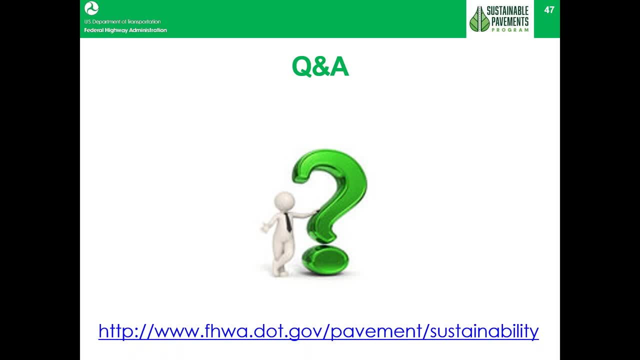 more of the statistical data that's involved with some of this if possible as well, so that you could do more probabilistic studies in the future on the LCA. But right now I do recognize that most of the studies in which wasn't mentioned today in environmental product decorations. 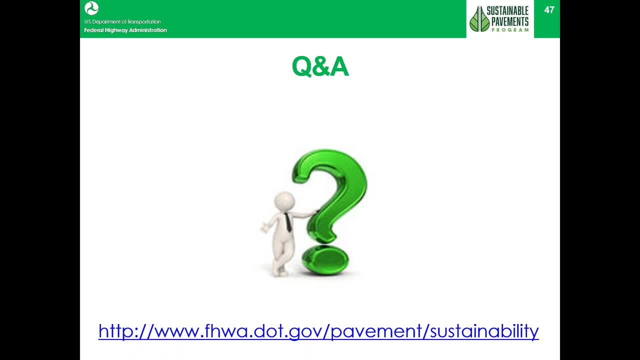 that's another data potential data source. they are just a deterministic value versus a value with some of the an average with some standard deviation. All right, Thank you, Heather. Let's go back to Misa. Misa, there was a question about 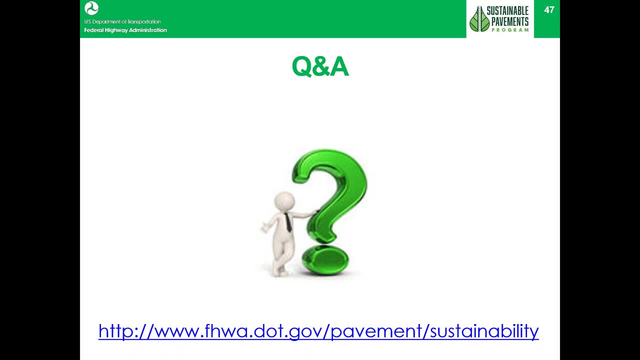 federal LCA commons and maybe you could talk a little bit more exactly what that is. Hi, sorry I was on mute. The federal LCA commons is the is a community of practice of LCA practitioners working with, in and for the federal government to align and advance LCA research. It also maintains: 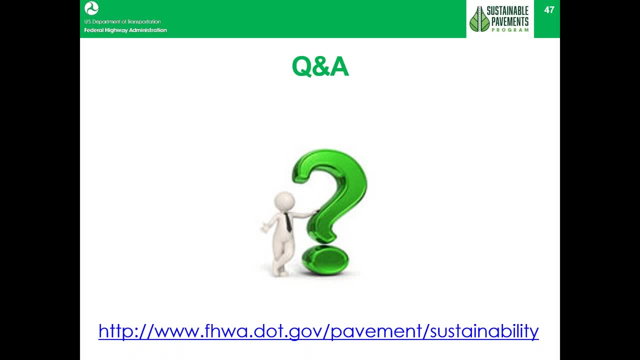 a repository dedicated to access to, and long term preservation of federal LCA data, tools and resources. Heather, aren't you on the LCA commons, or you were part of it at one point? Yes, We, so. FHWIA is a very important source for LCA research. 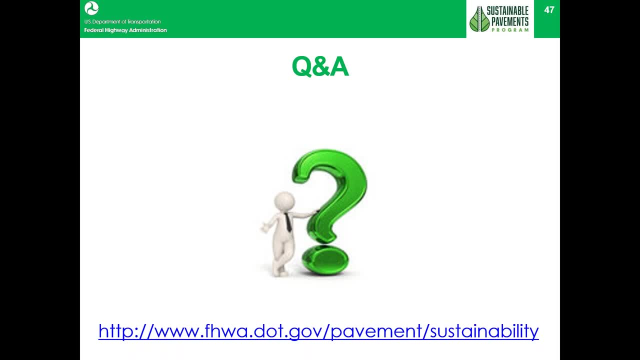 member of the, the federal lca commons, along with department of defense, usda, epa, the national labs, so argon, who is largely responsible for the greek models, as well as n-rail and many others, or nist mist, is involved, and so we're all trying to find synergies amongst our efforts and harmonize our 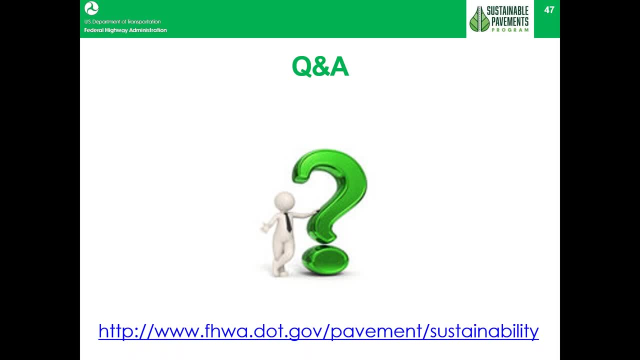 approaches um, and so one of the synergies that we found is we at fhwa with this group is we feel that there's a strong need for some common background data sets to help create epds that potentially could be used for public procurement, and so to do that, we're organizing the group to 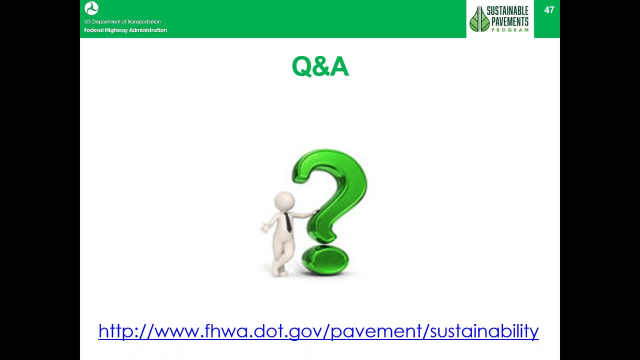 put together a road map towards background data sets, these common background data sets. there's been major efforts made towards a common electricity background data set that should be loaded on the repository soon, um, but we definitely need to tackle transportation, and that's where i think one of the previous questions as far as asphalt institute and the petroleum industry related to. 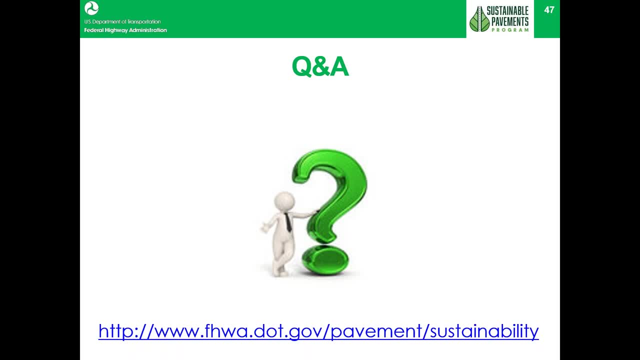 asphalt. there's a little bit of overlap and we'll have to work together um in in how we're going to harmonize that, um that, the transportation flow, and then the byproduct being asphalt from that stream. all right, great, thank you, heather um heather, as long as you're on the the line here, let's. 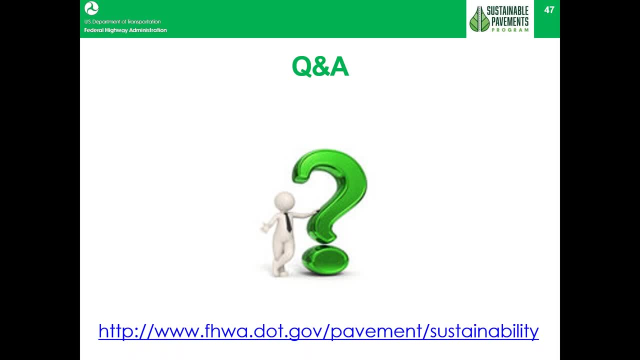 shoot another question your way. the question is: in doing a life cycle assessment, should you take into account a residual value when the service life extends beyond your analysis period, similar to kind of what's done on a life cycle cost analysis? say that again one more time. it helps. 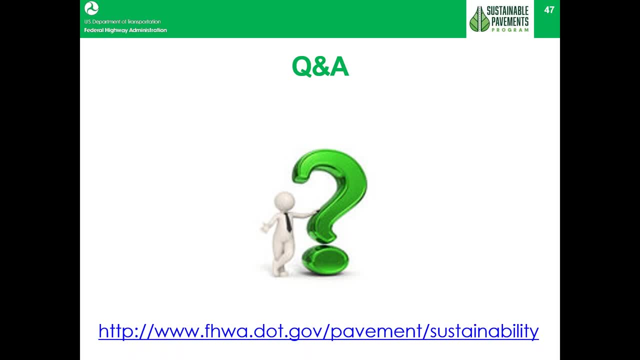 when i i'm reading them while you say, um, but i didn't catch where this one is on my list. so the question is like in life cycle cost analysis, where your service life extends- service life of one of your rehab treatments, for example, exceeds beyond your analysis period- you have a residual value that you account for that impact. 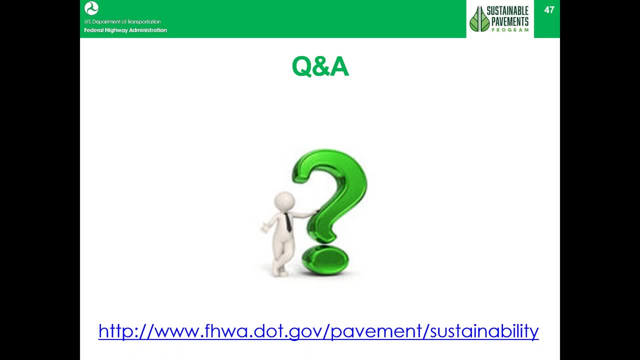 is a similar type of um factor needed in doing a life cycle assessment. yeah, so in the life cycle assessment you need to ensure that you have a functional unit and that the functional unit, if you're doing an attributional life cycle assessment where you're comparing one product to the other, the functional unit needs to. 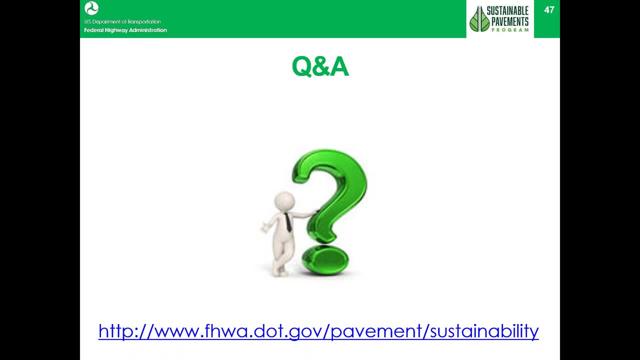 be the same, and so service life is particular, is usually part of that functional unit. and then you're absolutely correct: if one um has a longer service life than the other option, there are techniques that you can do to account for that, so that you are comparing apples to apples and the lca framework does give. 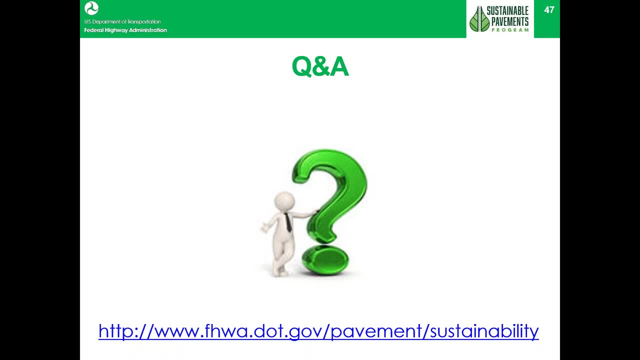 you some of those options. so if you do access the website and look at the federal highways life cycle assessment framework for pavements, it goes into some of the more details and strategies on how you would account for that. great, thank you. let's go back to um misa, uh misa. there's a question um other than illinois. 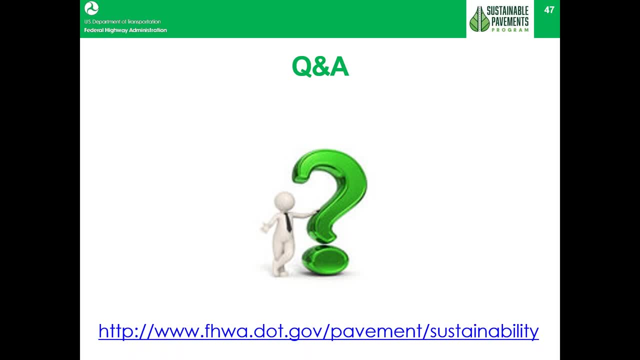 tollway and caltrans. are there any highway agencies or other other transportation agencies actively using life cycle or life cycle assessment in their decision making process? so i believe that the arizona department of transportation has started using life cycle assessment, um, but heather might know more about what other states are doing. 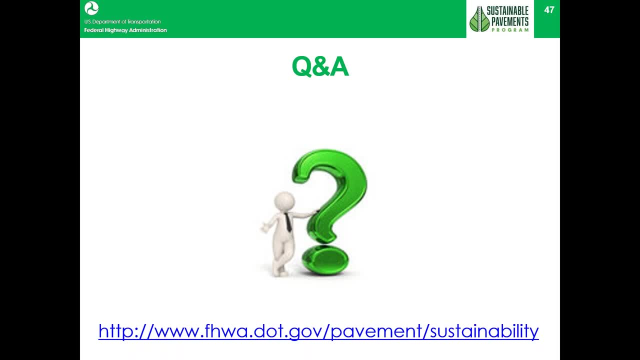 I'm not too sure. I know Hawaii is not, but there might be other states doing that. Yes, Misa, you're correct. Arizona State has shown interest. They haven't necessarily used LCA in their decision making, but they're definitely showing interest in learning how LCA could be. 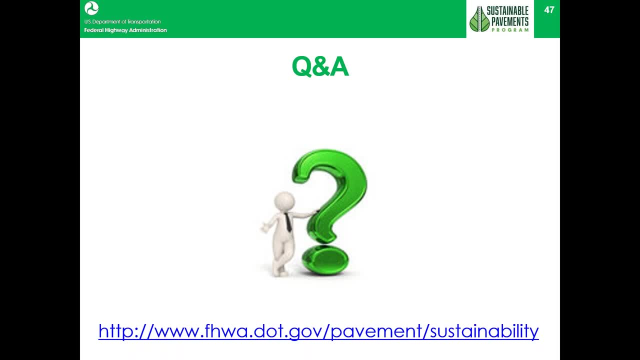 informative and used, And so I feel that they are one of our key champions. There are certainly other states that are being proactive in trying to figure out how LCA would be used at their agencies, largely trying to get ahead of current or proposed legislations that may be introduced. 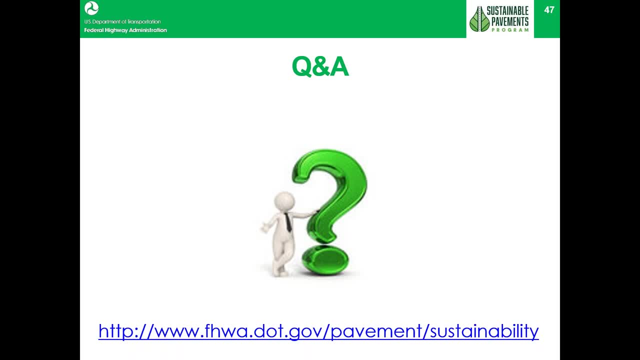 in their states, And so some of those states that have had recent legislations introduced or are suspecting that some would or could be introduced would be minority. Minnesota, Washington, Oregon, all have had some proposed legislation at the state level and in various drafts and versions, So they have been states that we've been working with. 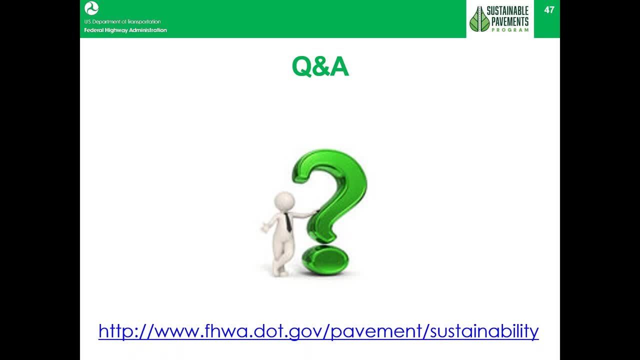 In addition, there's been some recent. I know in Oregon there is some recent, I think it's an executive order and push to reduce greenhouse gases. So I think Oregon DOT, you may be looking at LCA more from a programmatic approach on where are their hotspots, where they 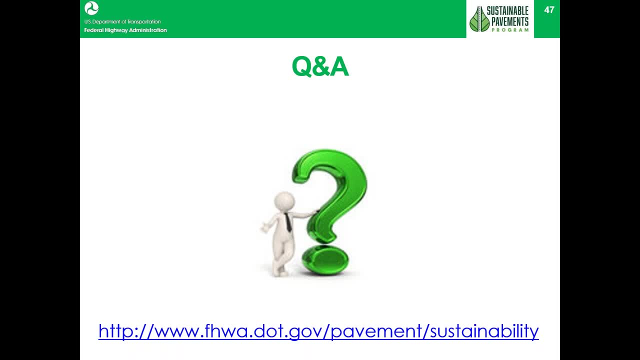 could look at reducing their greenhouse gas footprints. Maybe not specifically get to this design level, but due to that executive order, I know that there's some interest there, As well as what was some of the other states I think. I've seen benchmarks, similar type benchmark. 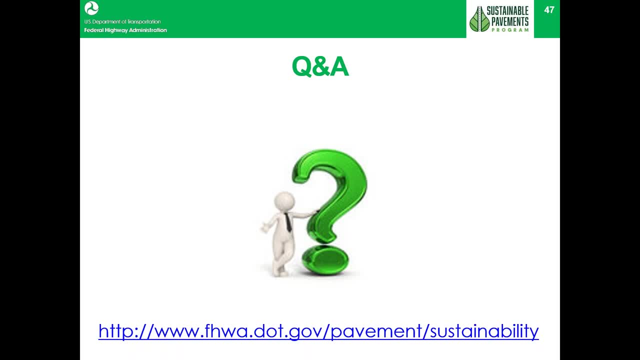 surveys out of Illinois. Sometimes the states may contract with a university to do some of these studies. So I think Illinois was contracted out to a university, but it was again more of where are the most of the embedded emissions, or embodied emissions, coming from in their purchasing. So again at the high level type. 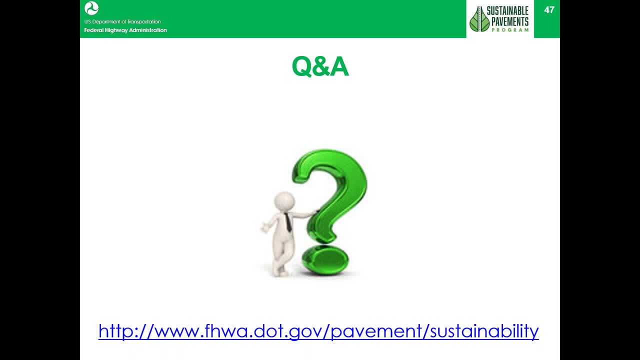 benchmarking, not in the pavement design aspect. All right, Thanks, Heather. And jumping over now on the topic of tools. there are several tools that were highlighted. They're just some general questions about the applicability of some of these tools. Are they? 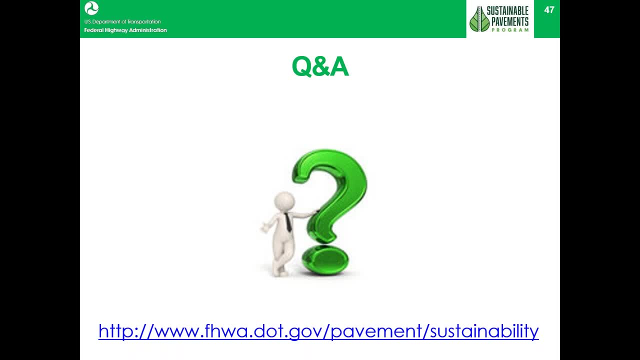 limited to use just in the US? Do they have international applicability? Maybe I'll throw that one to Heather Sure. All the tools are made with different purposes And you should always be aware of what went into the tool and what is some of the background. 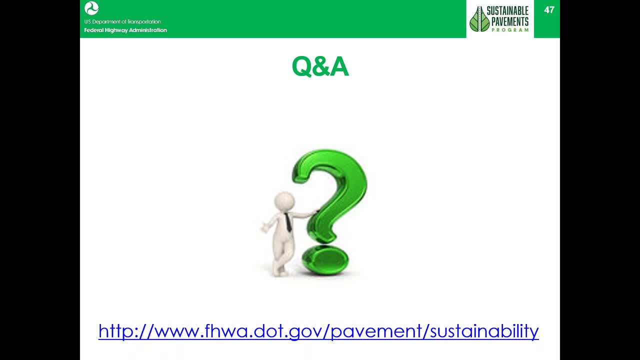 data and what is the goal and scope of how that tool was made for. And so, like I said, the FHWA tool is made specifically. the default data would be more geared towards the US, since it is for the be made by the federal highways from the US, So it wouldn't be. 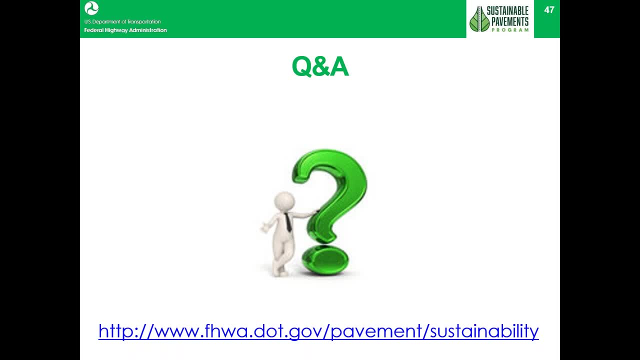 I think, necessarily made that would be applicable to other countries in the international sphere. but that doesn't mean that a lot of the framework that has been developed, especially a lot of the work that has been developed through the federal commons they're mapping out how the LCA should be done- couldn't be easily adapted for international. 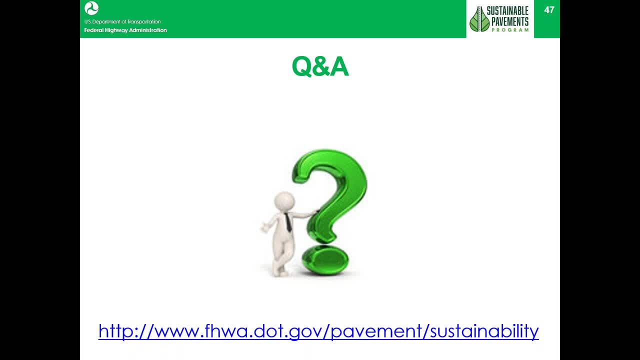 purposes. So the There are two efforts going on at FHWA and the LCA tool that was referenced by MISA that is going to be out in September is an Excel-based tool very similar to RealCost, And the one thing about that tool: you can add EPDs into it easily, and so you would be able to customize that tool to be used at an international level. 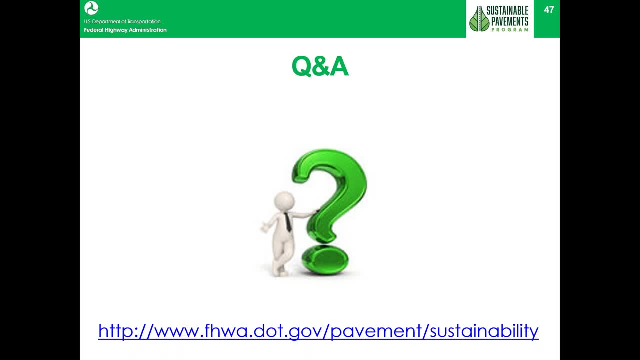 However, what I meant is the default data right now is geared towards the US, so you would have to do a little bit of work to take it and use. I'm not aware of any global pavement LCA tool that is applicable to all nations. 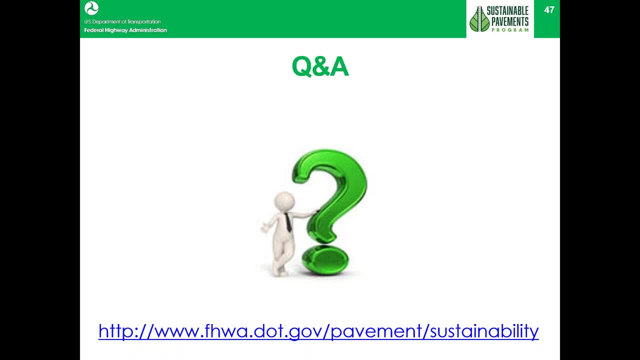 I am aware of European tools and France. they have one called SIV, Netherlands has one called DuoBookHawk. I think even there may be some in Sweden being developed, as well as Spain. So definitely Europe has a lot of activity in pavement LCA. 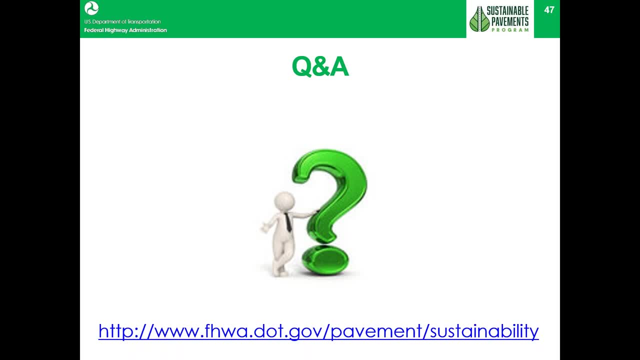 But with the second version of the tool that FHWA is working on with OpenLCA, we plan to map out all the unit processes that would go into an LCA and upload that framework in OpenLCA platform. So it's like taking that manual, the LCA framework that I referenced earlier. 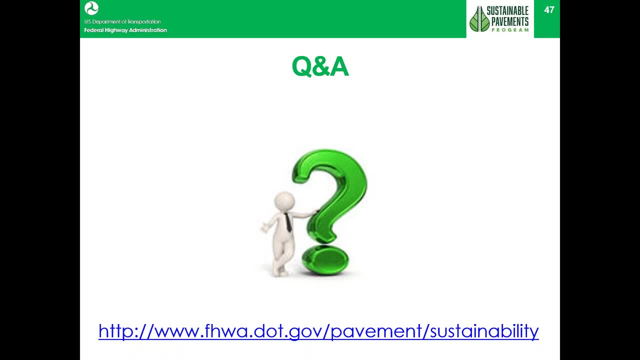 and actually Okay, And eventually putting it all together into an LCA software platform. That would be probably something that is the closest to a global tool and all you would have to do is update the data sets to the specific country, but it would have all the underlying framework mapped out in unit processes that is required. 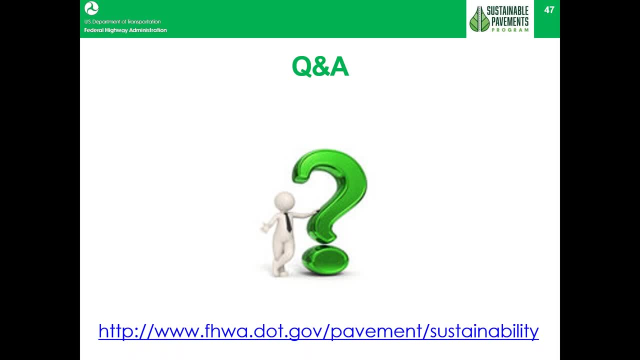 So it should be the Easiest to update. but that's more to support for future efforts in this program area. It's more advanced and hopefully in the future we could take the interface that's in the Excel tool and merge it with the OpenLCA platform and all that framework that we were being developed. 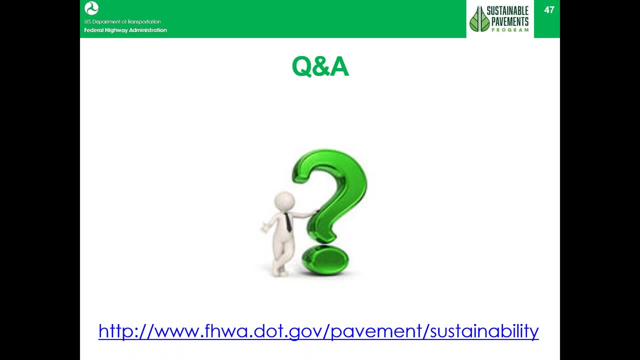 Okay, thanks, Heather. And coming back to you again still on the topic of Okay, thanks Heather. And coming back to you again still on the topic of Okay, thanks Heather. That seems to be a very popular issue right now. 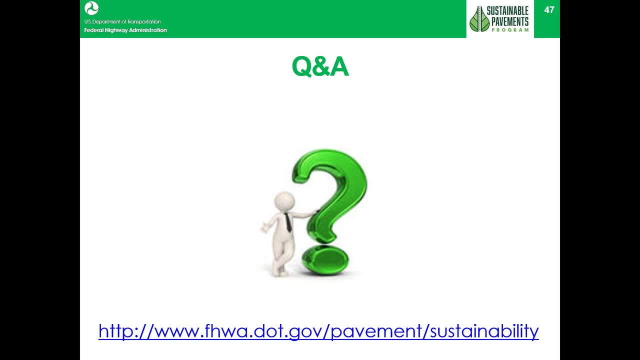 First of all, there's a question: whether you could provide a few more details about the FHWA Pavement LCA tool, maybe what it includes and whether or not it's an open-source software. So the Pavement LCA tool that we are creating in Excel, as I mentioned, is not open-source. 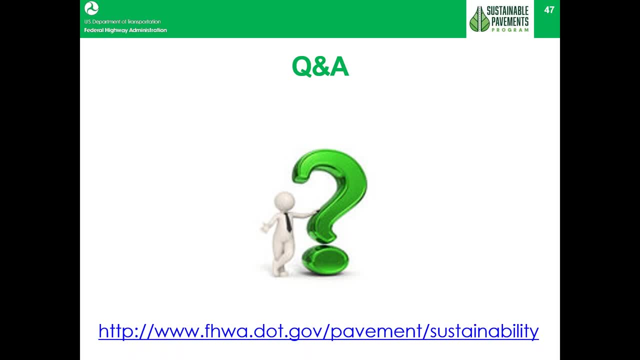 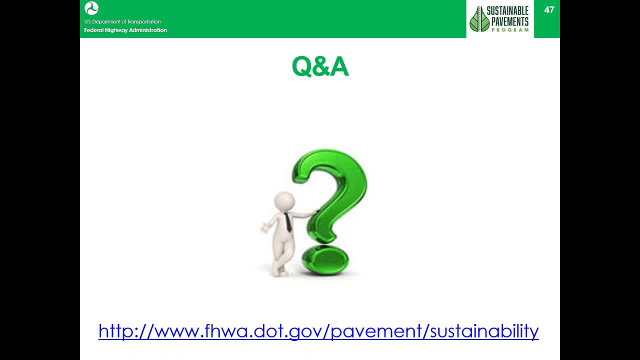 So we're going to have to do a little bit of a research on that. So we're just taking Excel and creating an interface to help facilitate with the calculations. Similarly, the other effort that I mentioned where we're mapping out the framework in OpenLCA. 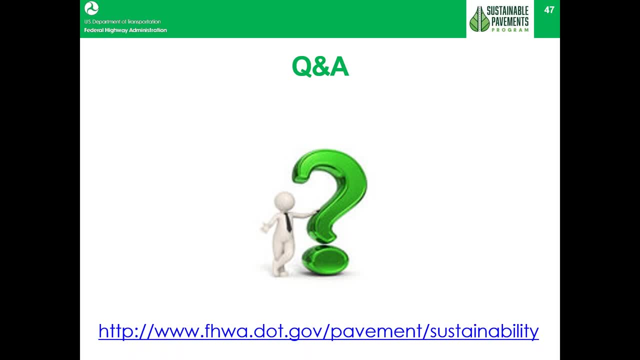 OpenLCA is an open-source software and there is a journal paper that's going to be published- hopefully in the near future, if it's not already- that explains the language language, the underlying language, to support further open source, the API for that particular. 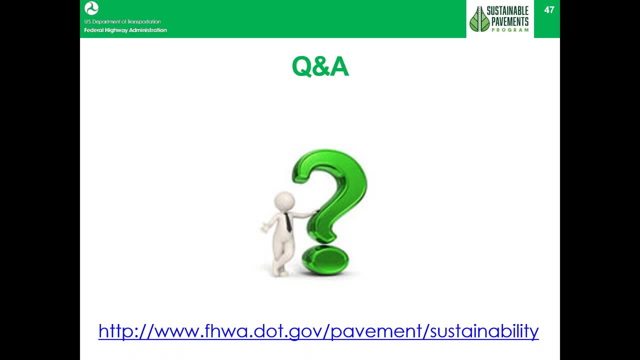 effort. So it is the closest thing to an open source nature that could be taken and made in that platform. But again, we're using OpenLCA, which is open source, and using that software to create the framework and added in the API that would be needed for pavements, pavement LCA. 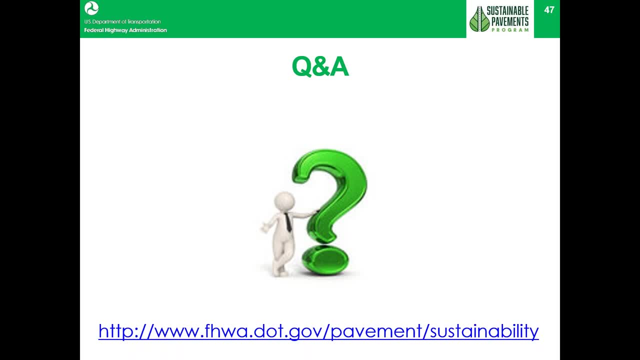 All right, And one more follow up, just on LCA tools. Are any of the currently available LCA tools capable of handling the use phase impacts? The one that I'm aware of that is available with the use phase is this, You know. 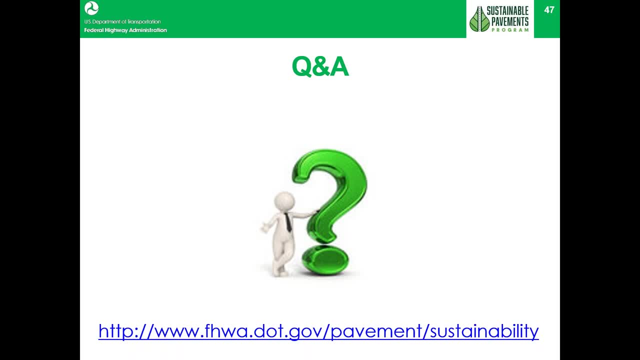 Yeah, This is a pavement LCA tool. As far as FHWA's stance on this is, we are currently have an effort that is looking at the use phase and particularly pavement vehicle interaction, And so we're trying to take this in a phased approach. 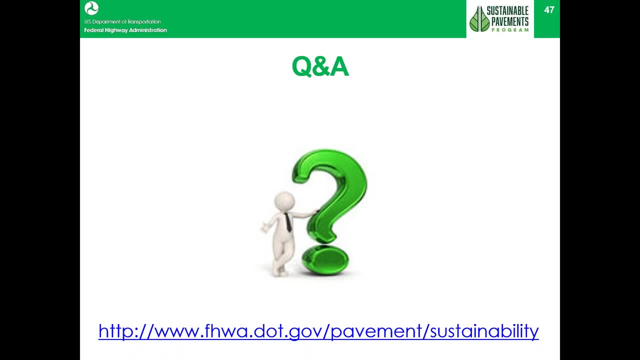 So we're starting with a simple It's cradle to grave in the fact that you can model the maintenance activities and the end of life activities In this LCA tool. however, we're not looking at the use phase as it pertains to urban heat. 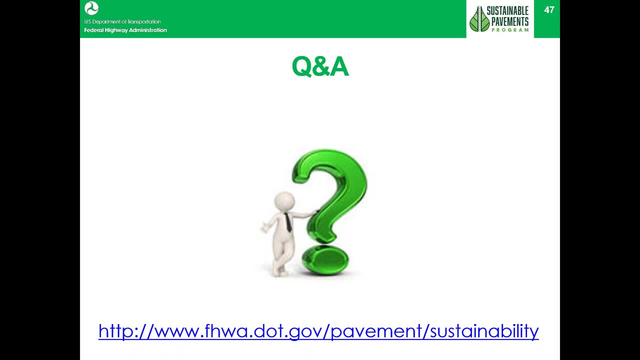 island issues as it pertains to stormwater runoff issues or your vehicle emissions, vehicle pavement, vehicle interaction and vehicle operating costs. So we're not looking at that yet And in the next phases of the tool and updates, That's something we would like to incorporate in in the future. 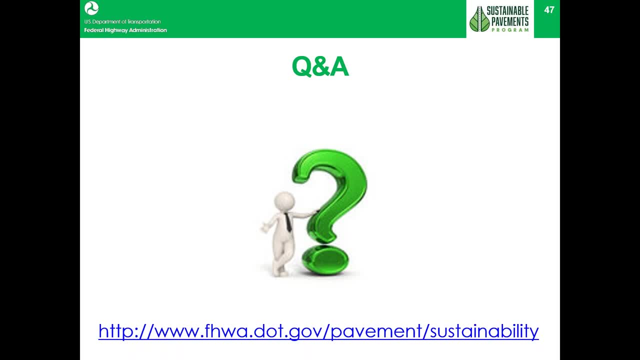 But, as I mentioned, we have another effort, that is, particularly looking at all the different models for pavement vehicle interaction and how easy and feasible are they to incorporate into LCA, or LCCA in that matter- to make decisions- And I don't think we're quite there yet- on what models we would recommend. 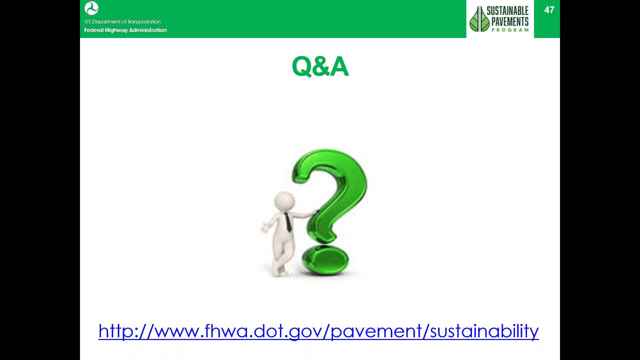 So that's where we stand there, All right, great. Thank you, Heather. Let's go back to Misa And Misa. there is a question of whether LCA can be applied to assess the environmental impact of different materials technologies, for example, the use of a recycled material. 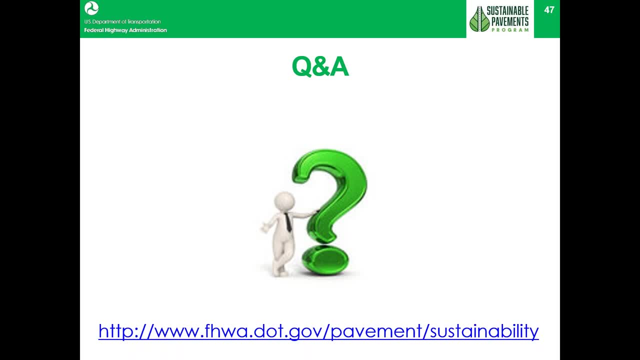 versus the use of virgin materials in, say, an asphalt mixture. Yeah, I believe that would be as part of the initial inputs for the raw materials that you would consider what the different inputs and outputs are from that individual material And that would also be part of your- probably your- pavement design. 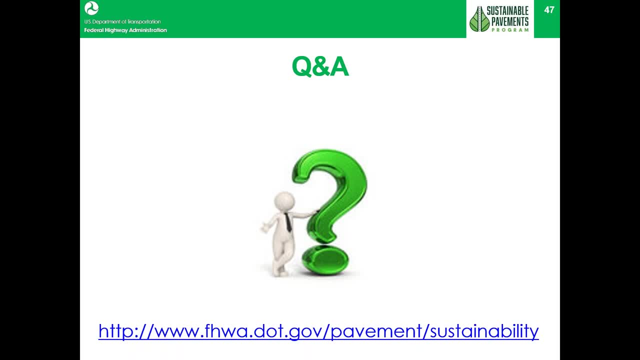 And then to manage the lack of field performance data. I mean you'd have to. that's probably one of the issues with, you know, adopting it for a specific agency or program is that the LCA needs to be tailored specifically to that agency and what the different parameters. 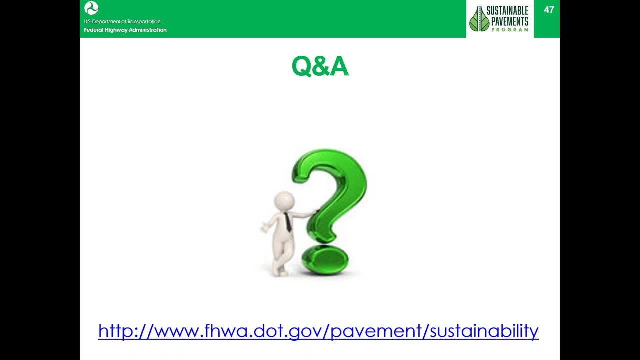 are. So if there's no data, that's where the data collection would have to come in, and you'd need to obtain quality data in order to get a quality LCA. But that's as far as my understanding. Maybe somebody else has a better answer. 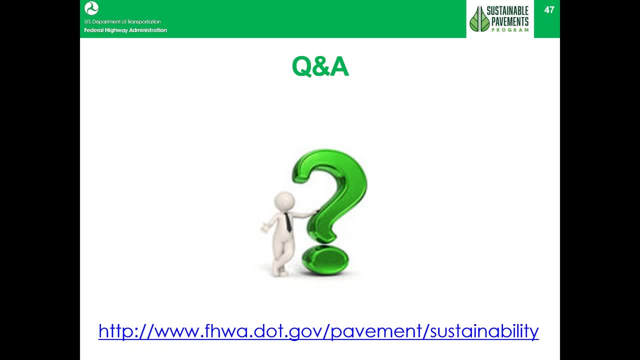 Anything to add to that? Heather, I think you're good. Yeah, you want, as far as performance, life. you'd want to know what you're comparing and use, If it's you know, repayment management systems. you could put this up in parallel to how you 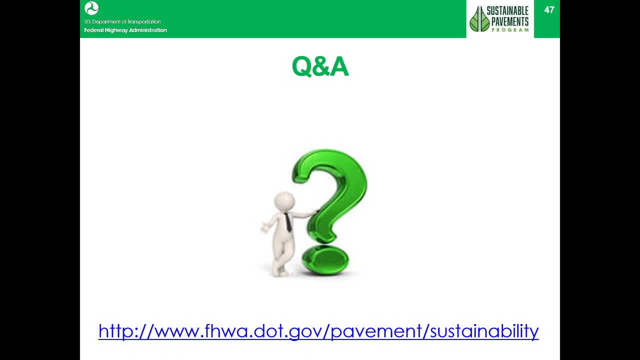 would conduct your LCCA, And so a lot of the inputs for your lifecycle cost analysis would be similar, other than how much materials are you using? that's a little bit different, All right, Another question. I think I'll pose this one to Heather. 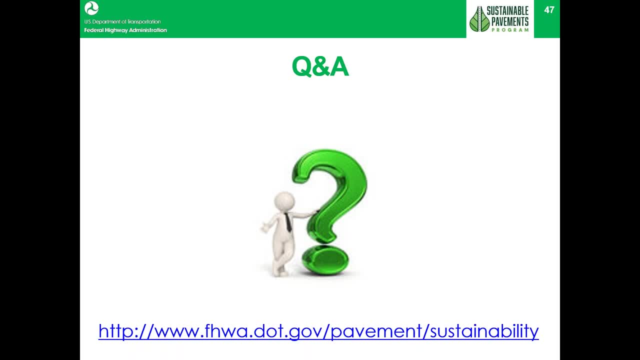 Heather the question. Heather the question. Okay, So the question is what precautions must be taken if the majority of the data available for an LCA is secondary in nature? So when you're using secondary data, that means you're using it a lot of the inputs. 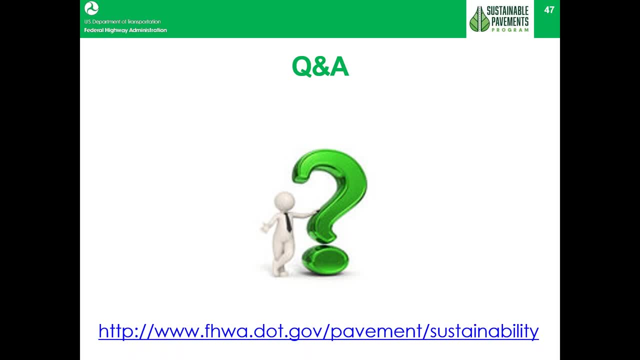 and the data is coming from some other source that may not be specific to what you're using. So you need to be careful. You need to be sure on the interpretation of your results are in line with the data sources that you have. And what I mean by that is if you're making a decision between a mixed design compared. 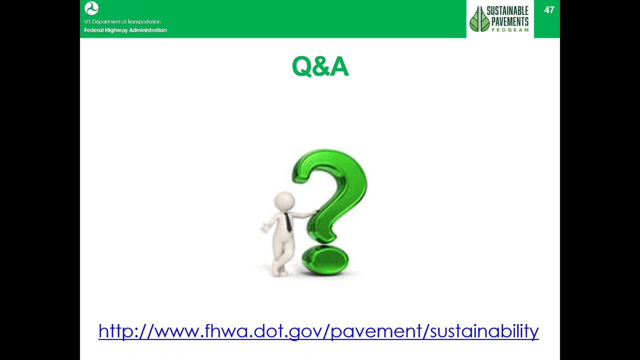 to another mixed design. you want to be sure that the differences in the actual results are coming from the differences in the mixed design, Okay, And not from these background data sets, potentially, So they should be in harmony. So what data needs you? what data you need for the study should be in line with your 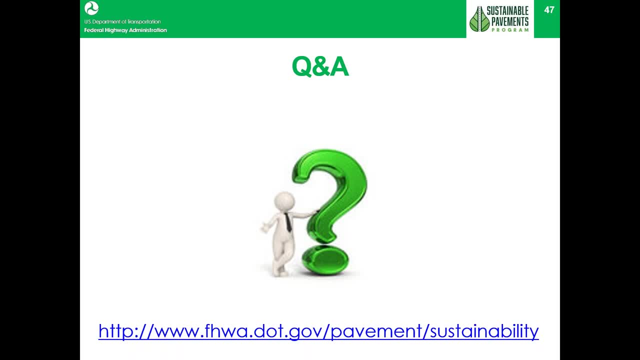 goal and scope And there may be a situation where you just don't have the data to use LCA to determine what you want in the end, and it is an iterative process. But there is statistical analysis that you can do And, as I mentioned, you know we want to push to get more statistical information and good 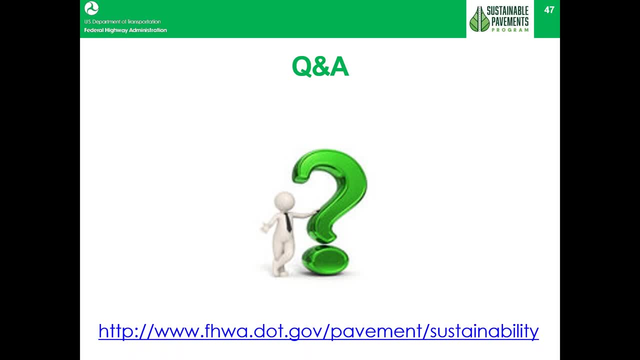 metadata and data quality on the background data sources, So we can use the statistical information in our LCA studies and do more of a probabilistic analysis, as we would recommend with lifecycle cost analysis. So I think that's it's evolution, you know, as we start looking at deploying LCA. 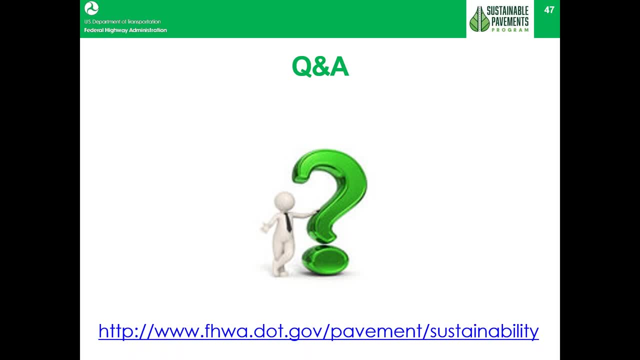 It's going to take some time. All right, thank you. Let's jump back to Misa Misa, the question about whether lifecycle cost analysis and lifecycle assessment should be used together. Is the goal to use those together as part of the decision-making process? 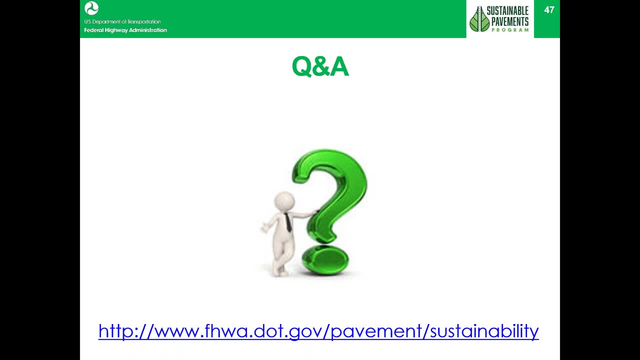 I think that would be up to what your priorities are in terms of you know benefits and costs of the different tools. So if you're considering you know more of your environmental impact versus more of your monetary impact, then that's where you would weigh those options of what you're going to. 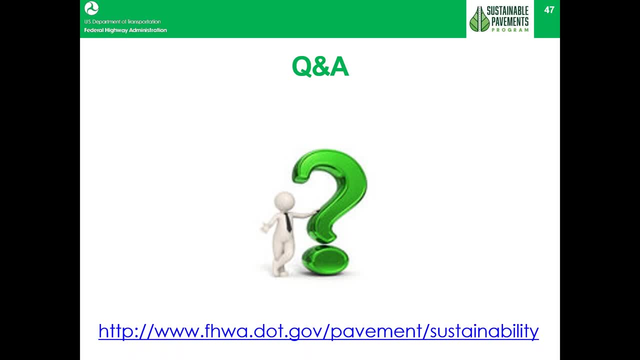 consider. But there are. you know that's up to the independent agency to make that decision on what they value, what they value the most out of those different measurements. All right, thanks, And kind of as a follow-up to that. 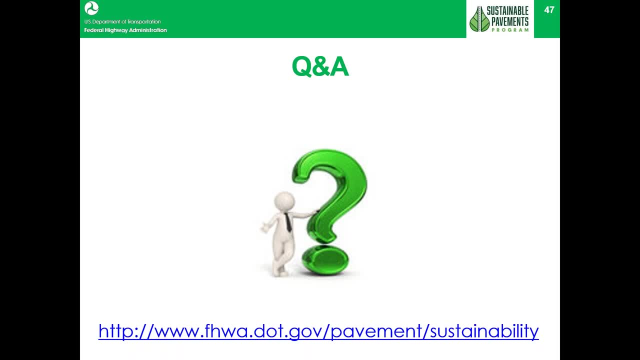 There's a question, A question of what is FHWA's perspective on LCA and how it would be used by an agency currently. Is it intended just kind of as an informational tool, or is FHWA looking eventually for it to be used as part of the procurement process? 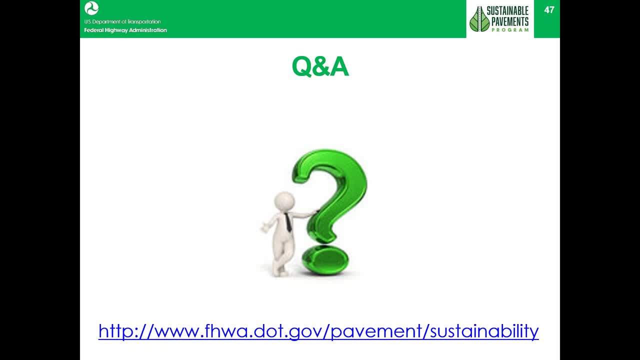 Go ahead, Heather. Yeah, I can answer that one Misa. I was going to chime in. I didn't realize He didn't direct it to anyone. He didn't direct it to anyone. So what we are recommending at FHWA is we're looking at LCA right now and trying to get 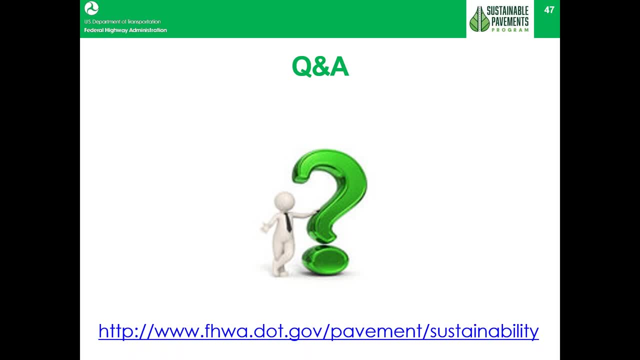 state DOTs engaged in understanding the LCA process, And so we're focusing primarily on education and outreach, largely because we're seeing that legislation is coming down and we would like agencies to be aware of what LCA is before prior to them being forced to have to do LCAs. 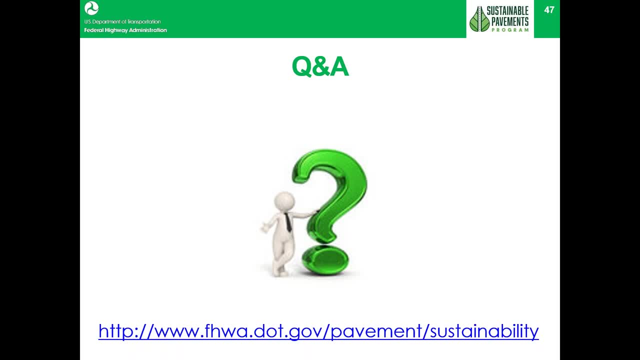 for every pavement design. In addition, though, I do see that the future of LCA would be to use it for decision-making, and it could be used in many different ways, And we have a paper that goes into LCA and how it can be used in your state transportation plans. 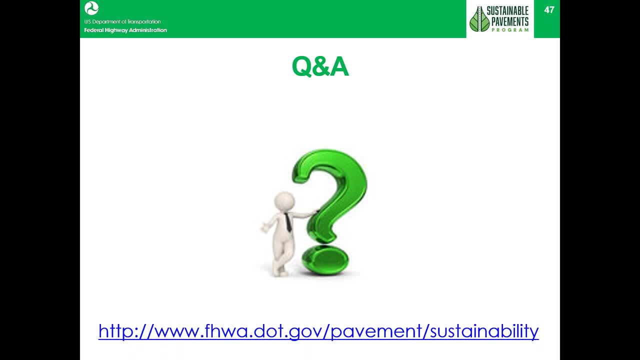 to the NEPA analysis and how it can later on be used in the bidding and then as built, and how you need to create feedback loops to transfer this data so that we're constantly informing all of those decision-making processes. So that's the end goal. 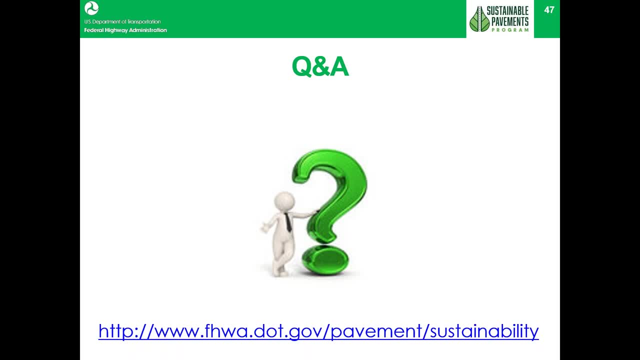 And so if you are signed up to our newsletters, which I assuming most of you guys are- if you aren't, I would encourage you to go on the website and become a friend. You'll get references to when that article is published and so that you could read and take a look. 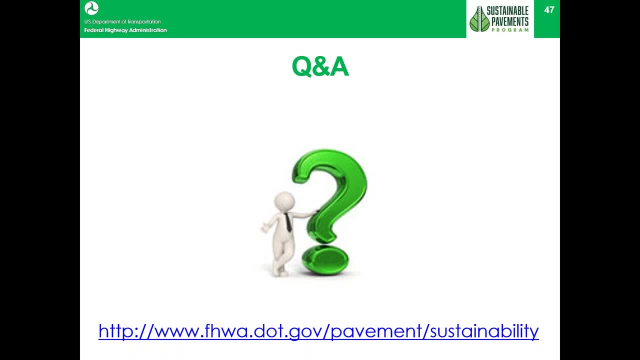 of how we see the future, What the future of LCA is in transportation and it's decision-making, But right now we're focused primarily on the education, building up the data. I think if you can build up and get good, solid data, 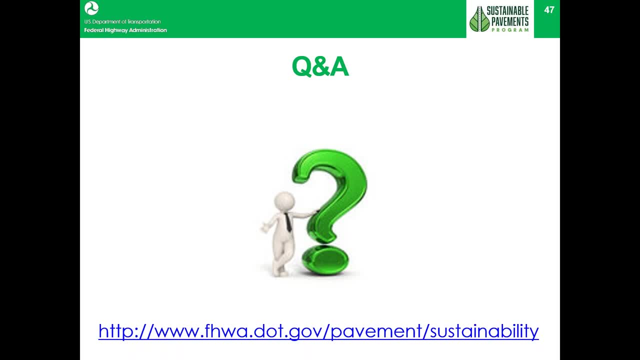 core background data sets that support industry EPDs, strong industry averages that can feed in to these LCAs. then we can use LCAs to build up, and then we can use LCAs in bidding or many different other applications. All right, thank you. 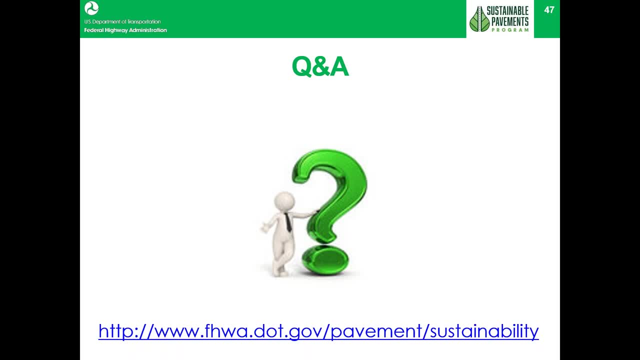 I'll direct this one to Misa Misa. there's a question about whether specific pavement techniques or treatments can be evaluated using LCA, And the specific example that the questioner raises is something like mechanical pavement. So, for example, mechanical stabilization using, say, geosynthetics. 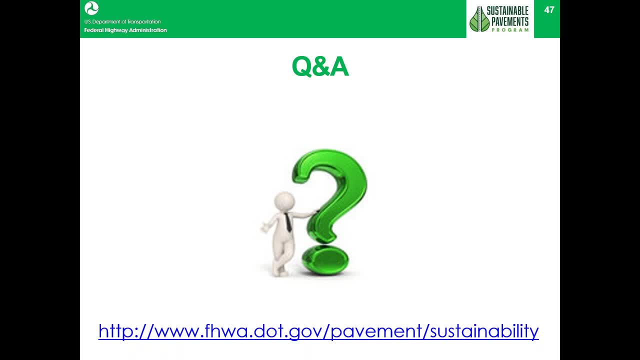 Is something like that capable of being modeled or considered in a life cycle assessment? I believe so. I think it considers the pavement design. So if you have instead of an eight inch base and then four inch overlay or asphalt thickness, then if instead you have something like TENSAR or whatever, 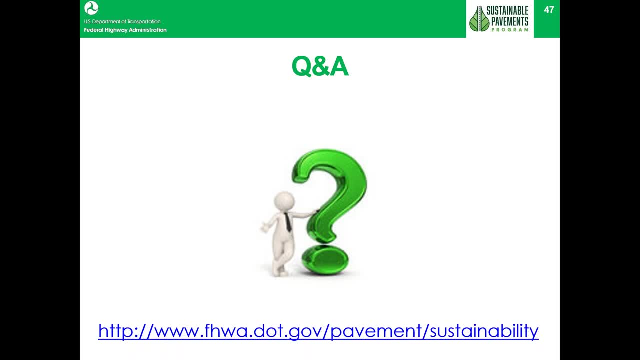 as part of the pavement design, then you can use it As part of your base stabilization. I think you would look at the different aggregate production and then also what's the production for that mechanical stabilization tool that you're using. So that's where you would have to compare. 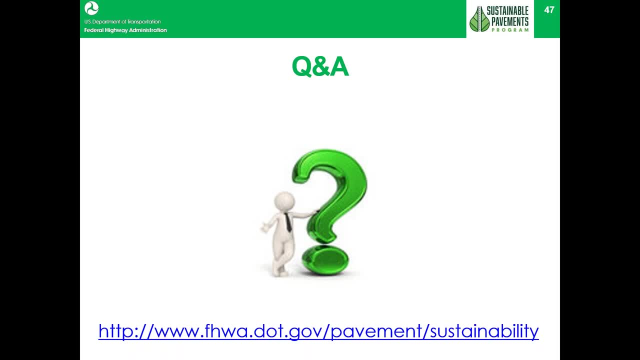 the different pavement designs that you can use Right and then be able to document the various environmental impacts associated with each of the different approaches. Yeah, and that's probably where the also like the life cycle cost analysis and stuff- comes in, and that's the considerations that you would be looking at. 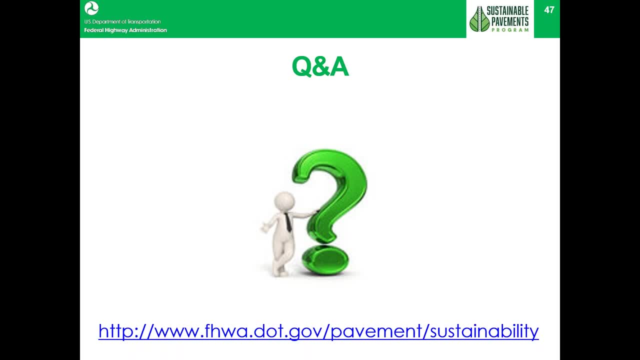 Right, all right. thank you, Heather. I'll turn this next one to you. Question is: if an agency wants to use a multi-attributed LCA indicator, has anyone estimated the relative weights of some of the different indicators? You know we don't have any recommended weightings as far as 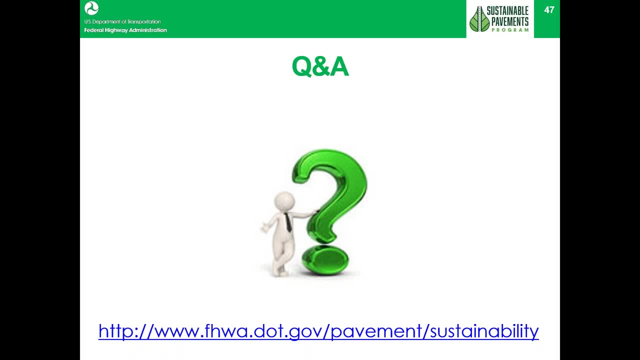 the federal LCA commons and work that we're doing- And I've heard that that was one of the needs or wants and desires of the federal LCA government, but heard that there may be some challenges in doing so, So I don't have anything to recommend. 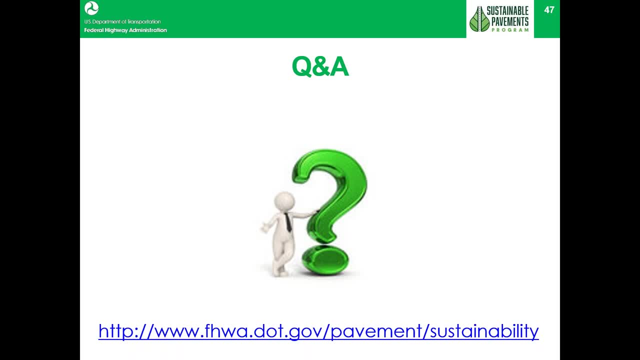 I do know that, at least in the past, there have been some weights included in some of the tools out of NIST that has in their birds and bees model And I think there's some testing models that looked at it and I think they used other scientific weightings. 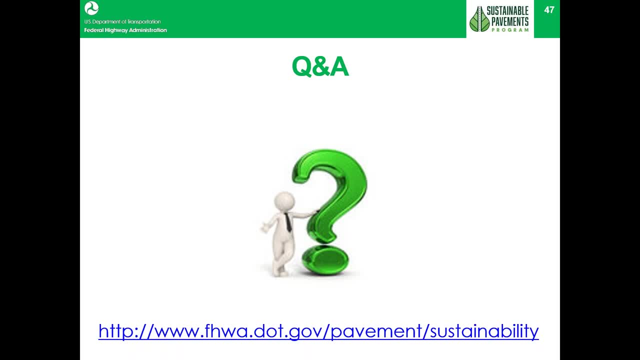 that had been done in the past, but they've never been updated for quite some time. So it is something that the federal LCA commons did discuss in our recent meetings, but I don't know if it's where we would be focusing at this point in time. per se. 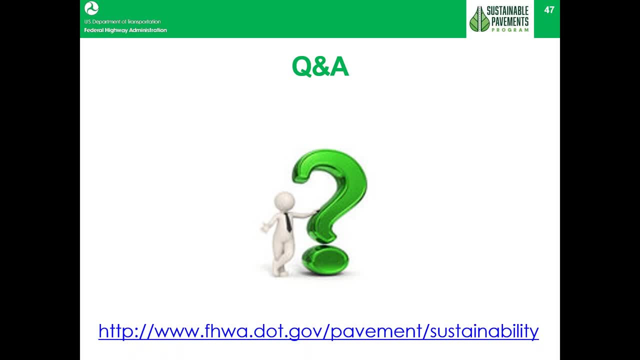 and we would be leaving it mostly up to the states to come up with their recommended weightings. All right, Thanks, And then I think we're down to just one final question. And, Heather, I think you kind of touched on this already, but if an agency is interested in starting, 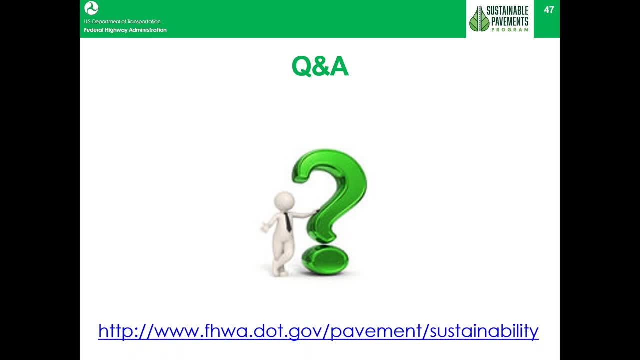 to get into this. where does an agency go to start getting data? Does FHWA have a database that may be available for use? So in our LCA tool, some data will be uploaded in there And then the agency, if they wanted to, they could start requesting EPDs and they 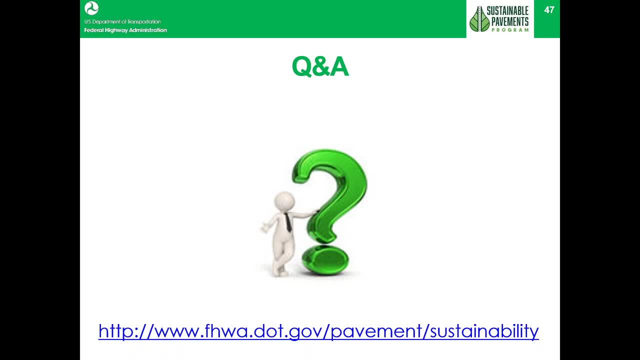 could potentially put EPDs up in there and start building even more data sets, But with regards to how to do that, I would really strongly encourage the agency to reach out to FHWA or Monica Geraldo, who's putting on this webinar series, And they can set up workshops. 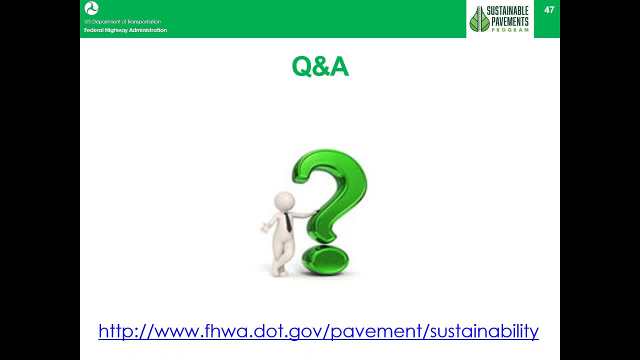 to help the agency To get started. we do have some one-pagers on the website, ones particularly for data and what are the data needs, because it is quite a data-intensive process And, as I mentioned, we are working in creating that roadmap for federal background data sets to start building.